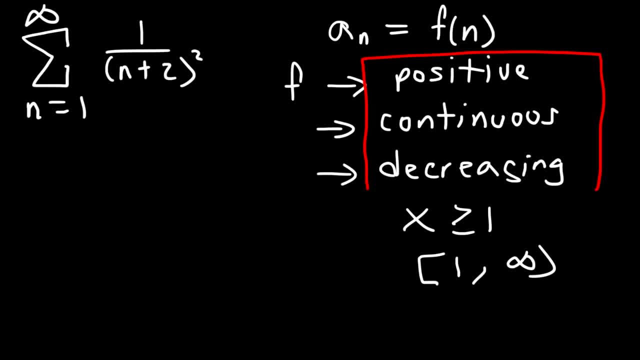 are satisfied, then we can use the integral tests. So here's the basic idea behind the integral tests: If you take the integral from 1 to infinity of f, of x, dx, and let's say you get a finite number which we'll call n, then the integral converges, which means that the series will also be convergent. 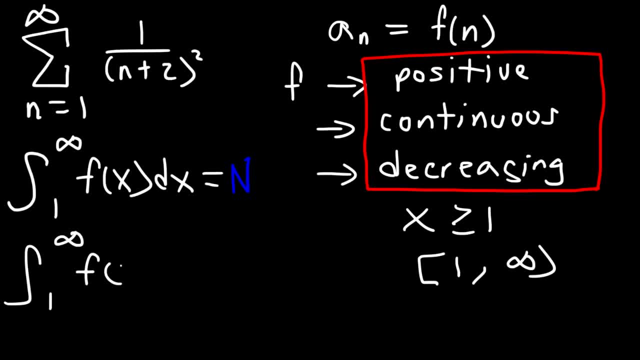 Now let's say, if you take the integral but you don't get a finite number, Let's say, if you get infinity or negative infinity, then the integral diverges. and so if the integral diverges, according to the integral tests, the series must also diverge. So that's the basic idea behind the integral tests. So now let's: 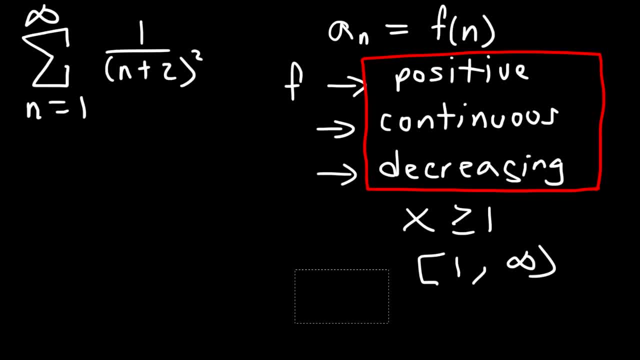 finish working on this problem. So let's write the corresponding function f of x, which is 1 over x squared plus 2 squared. So is this function positive? What would you say? We're looking at x plus 2 squared. Regardless of what value that we plug in, it's always positive, except when x is negative: 2. 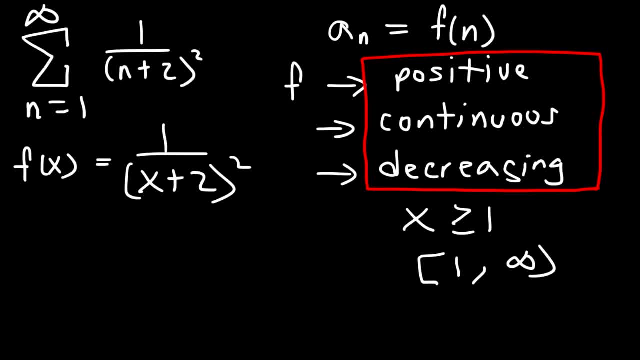 because we're going to have a vertical asymptote there. So for the most part this is a positive function. Now, is it continuous? Because we have a vertical asymptote at negative 2, that's basically an infinite discontinuity at that point. So it's not continuous everywhere. 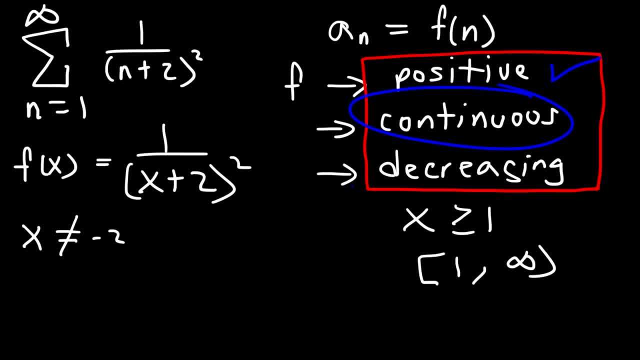 So does it satisfy this condition? Now remember it only has to be continuous on this interval and not everywhere. So is this a negative function? No, it's not. So does it satisfy this condition? No, it's not. This continuity, is it in the interval? Negative 2 is not in the interval. 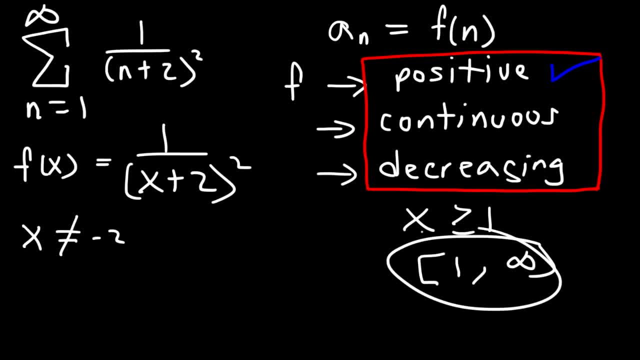 So, from 1 to infinity, it's continuous everywhere in this interval. Therefore, the second criteria has been satisfied. Now let's focus on the third point. Is the function always decreasing? The way we can determine that is by taking the first derivative. 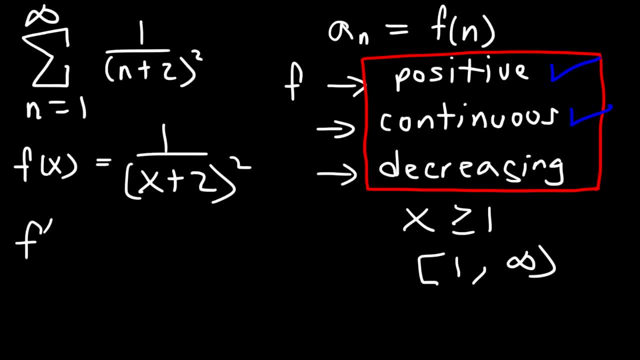 or using the first derivative test. If the first derivative is negative, then the first derivative is negative. If the first derivative is negative, then the function is decreasing. So we need to show that the first derivative is negative on this interval. So let's go ahead and find the first derivative. 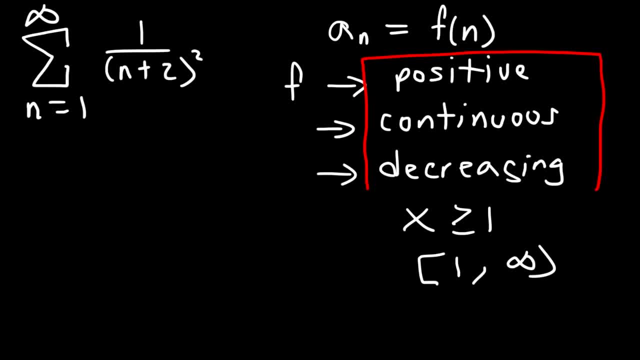 are satisfied, then we can use the integral tests. So here's the basic idea behind the integral tests. If you take the integral from 1 to infinity of f, of x, dx, and let's say you get a finite number which we'll call n, then the integral converges, which means that the series 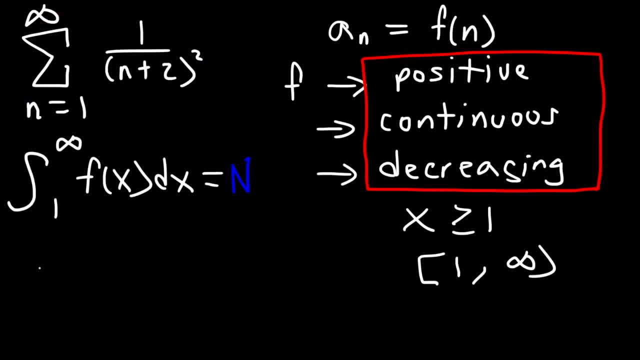 will also be convergent. Now let's say, if you take the integral but you don't get a finite number, let's say, if you get infinity or negative infinity, then the integral diverges. And so if the integral diverges according to the integral tests, the series must also 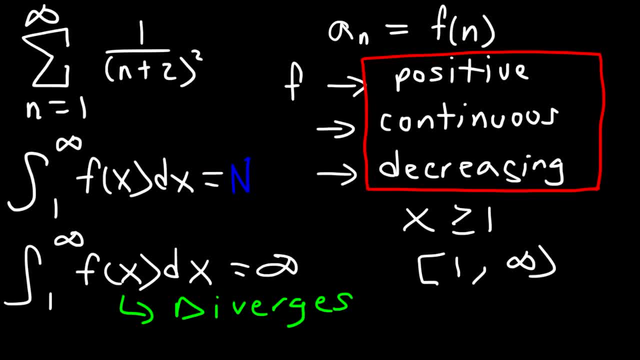 diverge, And so that's the basic idea behind the integral tests. So now let's finish working on this problem. So let's write the corresponding function, f of x, which is 1 over x squared. So f of x squared is the integral of x plus 2 squared. So is this function positive? 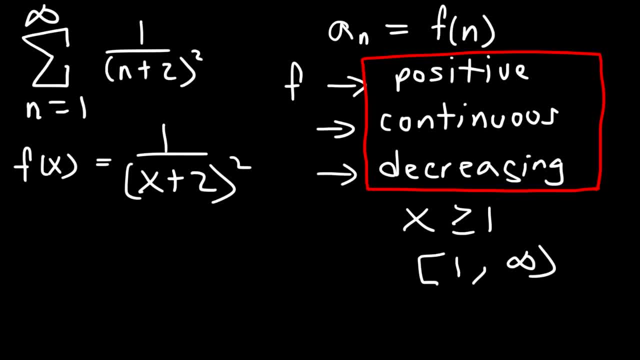 Or what would you say? Well, looking at x plus 2 squared, regardless of what value that we plug in, it's always positive, except when x is negative 2, because we're going to have a vertical asymptote there. So for the most part, this is a positive function. Now is 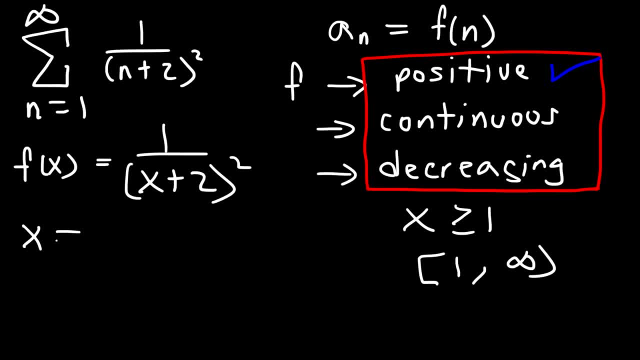 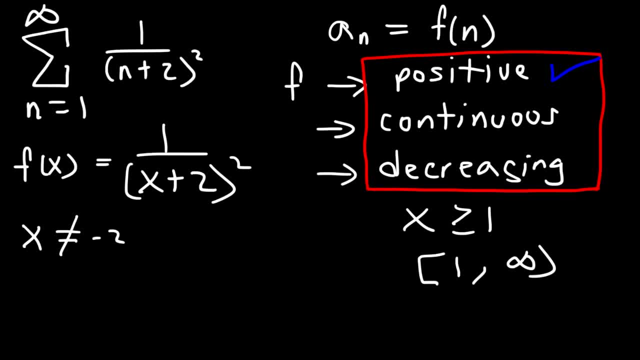 we're going to have a negative asymptote, And so we have a positive asymptote, And so we're going to have a negative asymptote, And so all of this is like this Positive شهداء to infinity. it's continuous everywhere in this interval. therefore, the second: 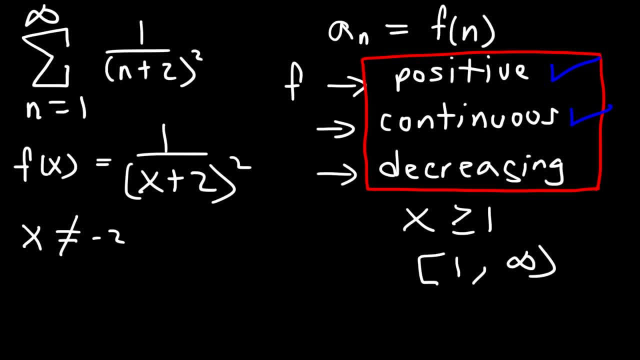 criteria has been satisfied. now let's focus on the third point. is the function always decreasing? the way we can determine that is by taking the first derivative. we're using the first derivative test. if the first derivative is negative, then the function is decreasing. so we need to show that the 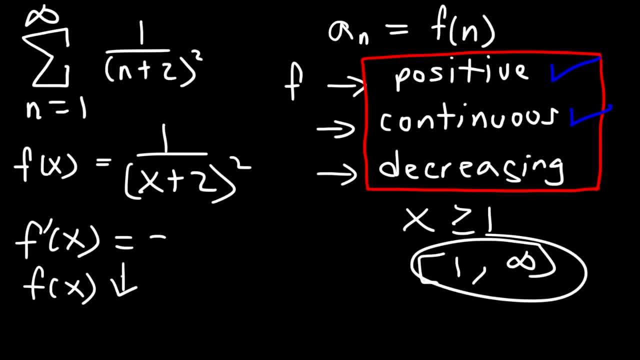 first derivative is negative on this interval. so let's go ahead and find the first derivative. so let's begin by rewriting it as X plus 2 raised to minus 2, and now let's take the first derivative of that function. so using the power rule, it's going to be negative 2 times X plus 2 and then negative 2 minus. 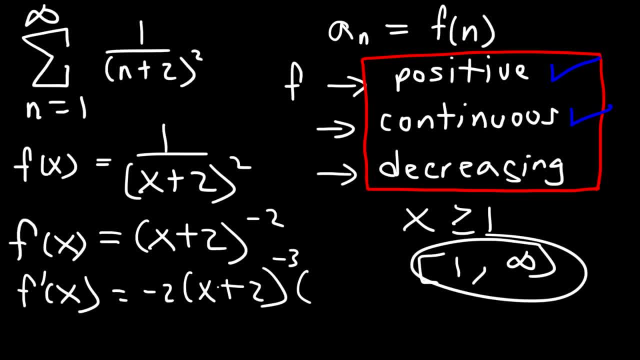 1 is negative 3. and then you need to multiply by the derivative of the nested function, which is 1. so we write in: this is going to be negative 2 over X plus 2 to the third power. so, looking at f prime of x, what can you tell me about the first derivative, about 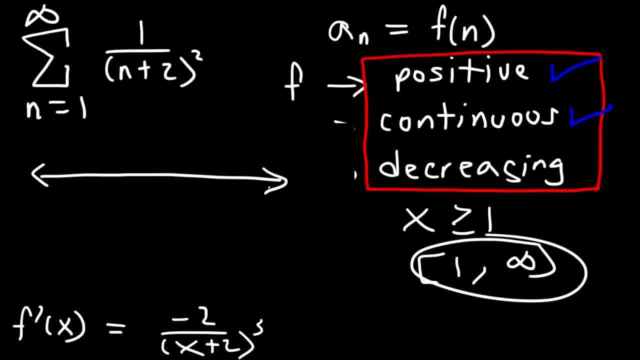 the sign of the first derivative. well, let's make a sign chart. so we still have a point of discontinuity at negative 2 and at that point it can change sign. so let's say if we plugged in negative 3, negative 3 plus 2 is negative and it's raised to the third power. so it's going. 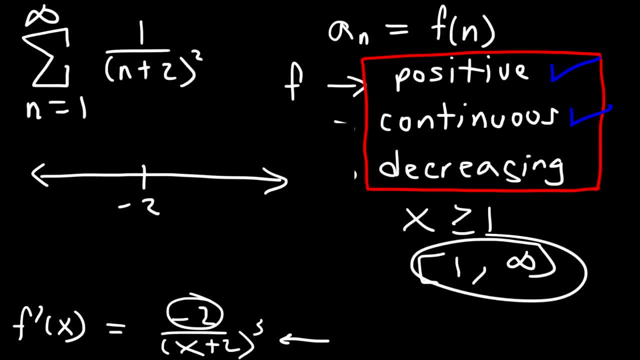 to stay negative, and a negative divided by negative will give us a positive value. now, if we plug in a number that's greater than negative, 2, like the 0 and 0 plus 2, is positive. so a negative number divided by a positive number will. 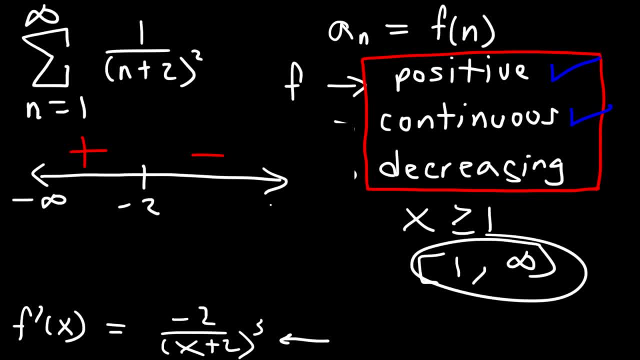 give us a negative result. so from negative 2 to infinity, the first derivative is negative, which means that the function f of x is decreasing. so if it's decreasing from negative 2 to infinity, it's also decreasing on the interval from 1 to infinity, and so that's one way. 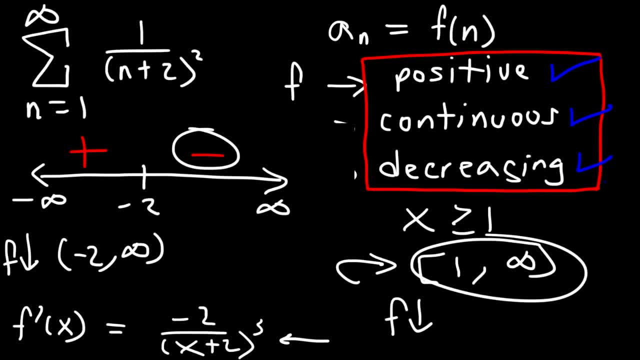 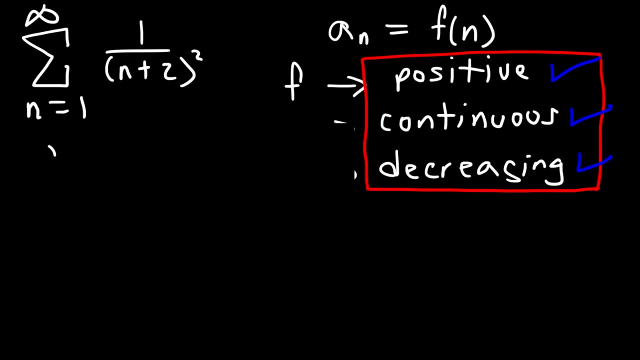 you can show that the function is decreasing on this interval is by taking the first derivative and making sure that the first derivative is negative on that interval. so once you show that the three conditions are satisfied, you can now use the integral tests. so let's evaluate the integral from 1 to infinity. 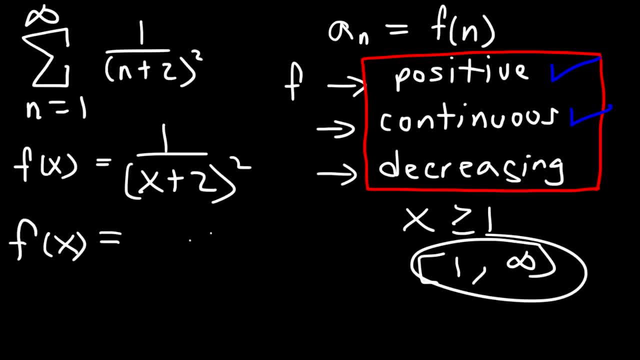 So let's begin by rewriting it as x plus 2 raised to minus 2.. And now let's take the first derivative of that function. So, using the power rule, it's going to be negative 2 times x plus 2, and then negative 2 minus 1 is negative 3.. And then you need to multiply the 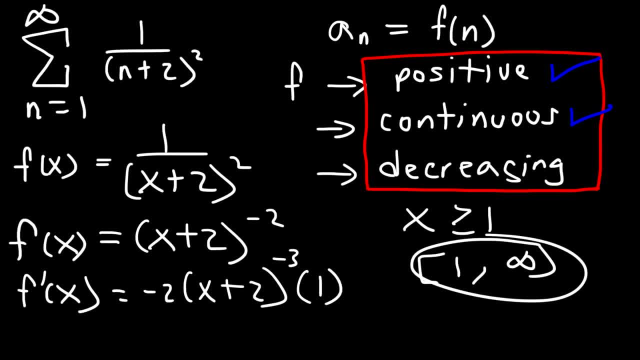 derivative of the nested function, which is 1.. So rewriting this is going to be negative 2 over x, plus 2 to the third power. So, looking at f, prime of x, what can you tell me about the first derivative, about the sign of the first derivative? Well, let's make a sign chart. 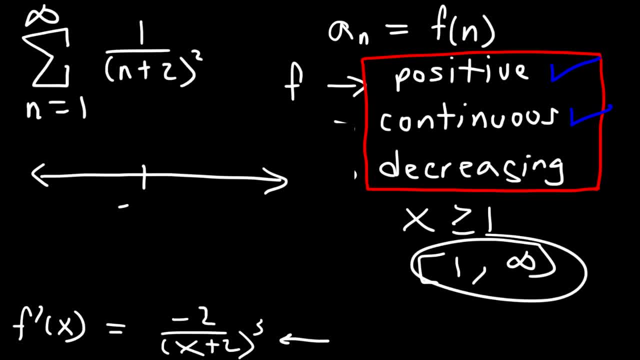 So we still have a point of discontinuity at negative 2. And at that point it can change sign. So let's say, if we plugged in negative 3. Negative 3 plus 2 is negative and it's raised to the third power. so it's going to stay negative And a negative divided by 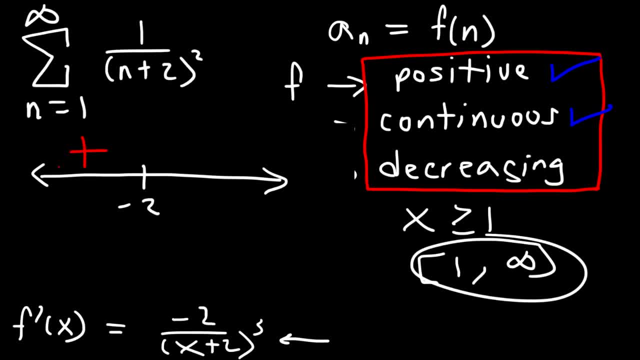 a negative will give us a positive value. Now, if we plug in a number that's greater than negative 2, like the 0, and 0 plus 2 is positive. so a negative number divided by a positive number will give us a negative result. So, from negative 2 to infinity, the first. 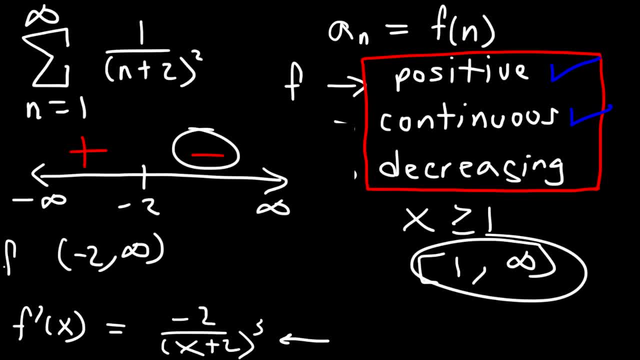 derivative is negative, which means that the function f of x is decreasing. So if it's decreasing from negative 2 to infinity, it's also decreasing on the interval from 1 to infinity, And so that's one way you can show that the function is decreasing on its interval. 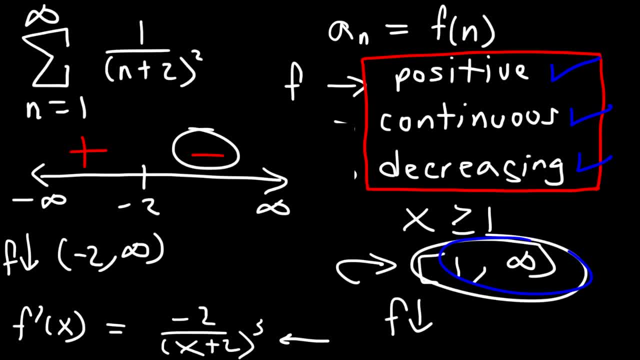 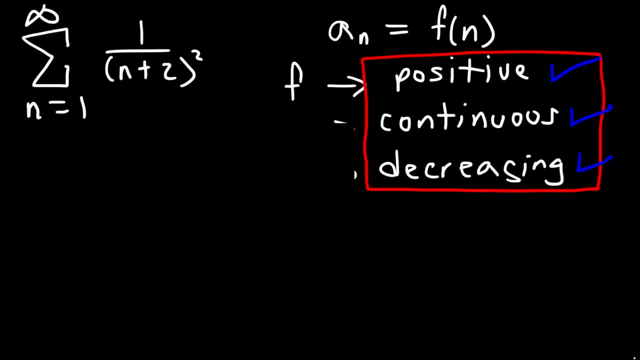 By taking the first derivative and making sure that the first derivative is negative on that interval. So once you show that the three conditions are satisfied, you can now use the integral test. So let's evaluate the integral from 1 to infinity of the function f of x, dx. So 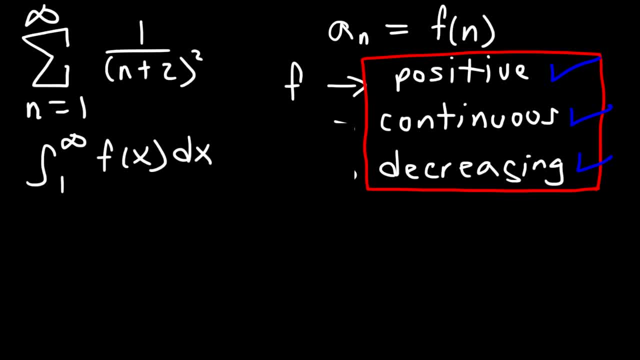 of the function f of x, DX. so this is an improper integral. so we need to set it up this way. let's use b, the limit, as b approaches infinity by itself, subdivided by 2 times 있는 Subtitle Me, infinity from 1 to b. and then f of x is 1 over x plus 2 dx. So at this point I can. 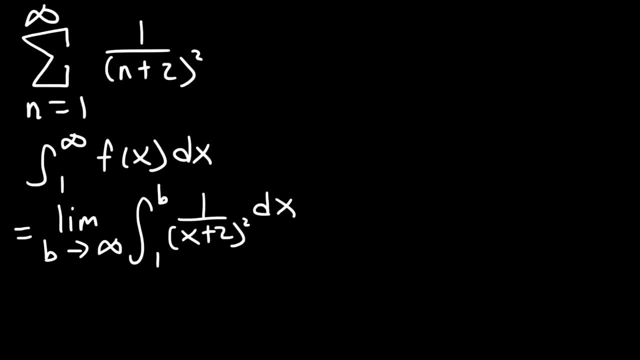 get rid of this stuff. We don't need that anymore, So let's focus on this integral. Now we can come back to this expression. So we need to do u substitution. So let's make u equal to x plus 2, and so du is equal to dx, So we have the integral from 1 over. 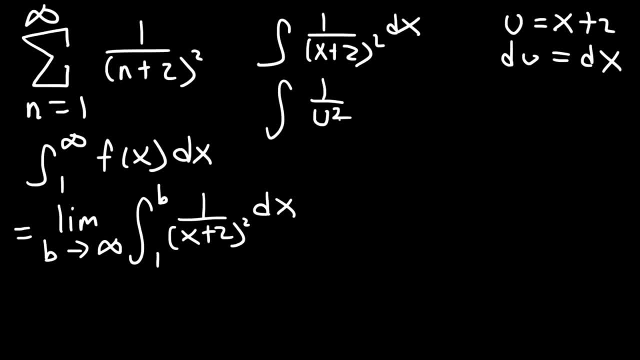 u, and then actually it's 1 over u squared times du. So we can write it as u to negative 2, and then, using the power rule for integration, negative 2 plus 1 is negative 1.. And so this: 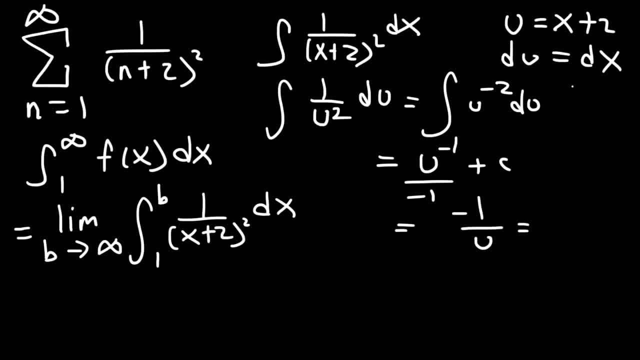 is going to be negative 1 over u and then replacing. we really don't need to see here replacing u with x plus 2.. It's going to be negative 1 over x plus 2.. So this is going to be equal. 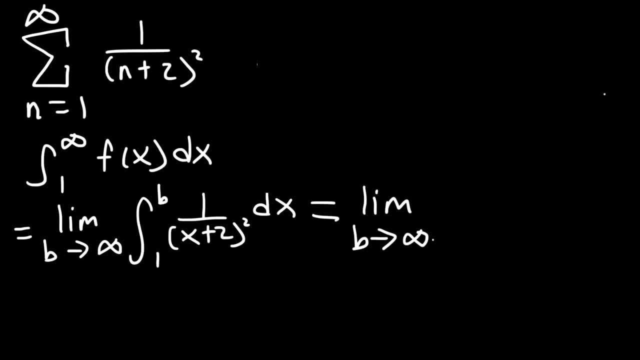 to the limit as b approaches infinity, and then this integral is going to be negative: 1 over x plus 2. Evaluated from 1 to b. So we're going to have the limit as b approaches infinity, and then we're going to plug in b into this expression. So it's going to be negative: 1 over b plus. 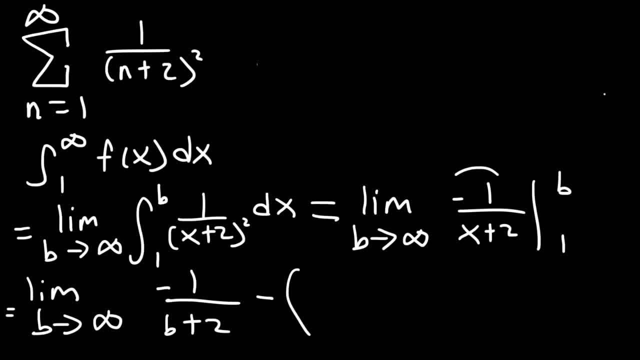 2, and then minus. now we need to plug in 1, so it's going to be negative 1 over 1 plus 2, which is 3.. Now the limit as b approaches infinity for negative 1 over b plus 2, that's. 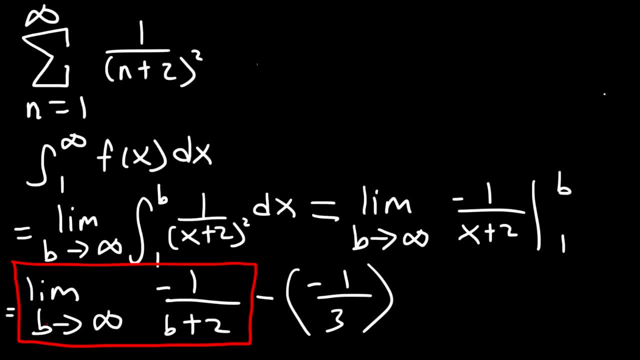 going to go to 0. If it was 1 over b, that will go to 0 as well. so negative 1 over b plus 2, that's also going to go to 0.. And then we have minus negative 1 third. so this is going to be plus 1 third. 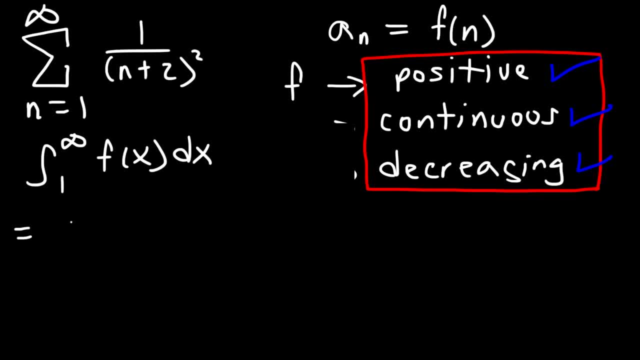 this is an improper integral, So we need to set it up this way. Let's use b, The limit, as b approaches infinity, from 1 to b, And then f of x is 1 over x plus 2 dx. So at this point I can get rid of this stuff. We don't need that anymore. 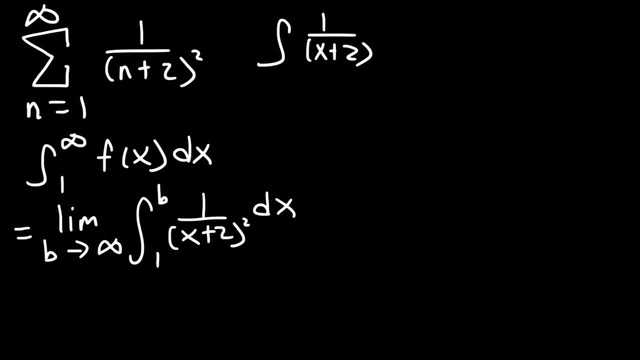 So let's focus on this integral And we can come back to this expression. So we need to do u substitution. So let's make u equal to x plus 2. And so du is equal to dx, So we have the integral from 1 over u. 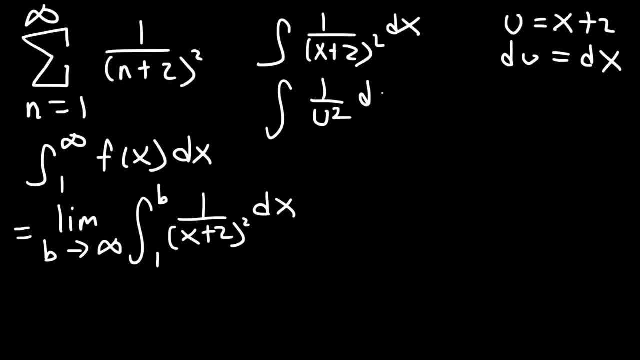 And then actually it's 1 over u, squared times du, So we can write it as u to negative 2.. And then, using the power rule for integration, negative 2 plus 1 is negative 1.. And so this is going to be negative 1 over u And then replacing. we really don't need to see here. 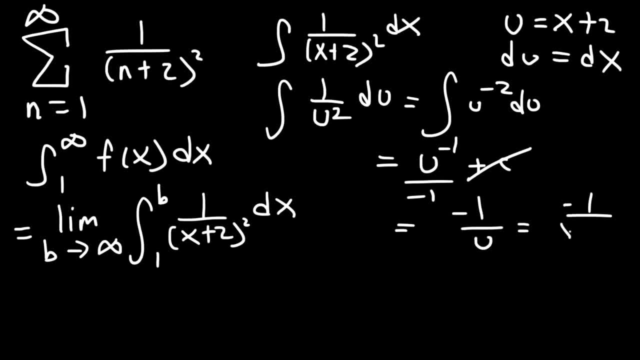 this is going to be negative 1 over x plus 2.. You can pick any one of these variables that works well for you guys. Now to define a solution for u. it's going to be negative 1 over x plus 2.. 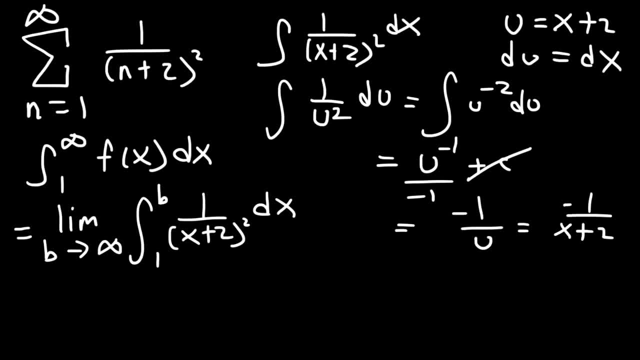 So you get negative 1 over x, plus 1 divided by a value. But since I already said that u is equal to the next one, If we multiply it by the definite value of u over y, you'll see that now we have the. 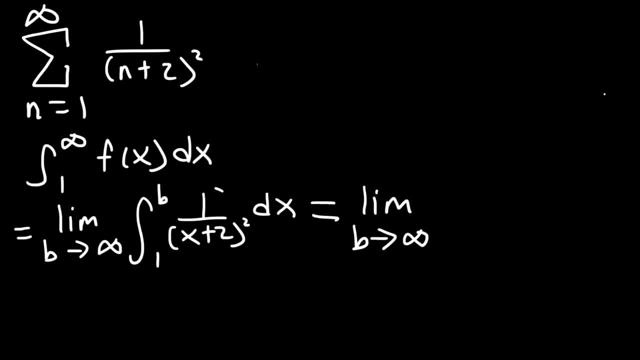 entire dimension. So let's address b this way. Let's circle it. This is like e prime multiplied by 0, and after that you can me this volume by neica prime multiplied by n. This is inside Bu. Alright, so that's AAä goof. 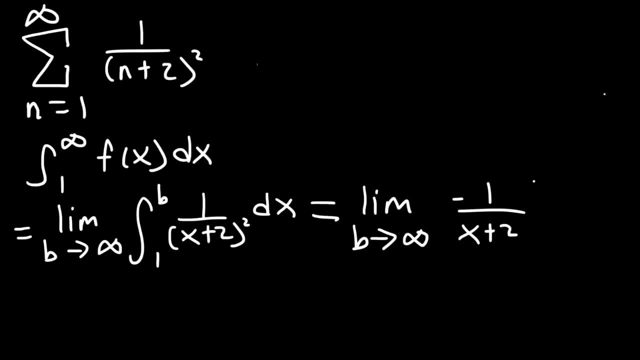 Alright, now let's imagine that U is maximum, So let's make u 0.. 2 evaluated from 1 to b, So we're going to have the limit as b approaches infinity. and then we're going to plug in b into this expression, So it's going to be negative 1 over b plus. 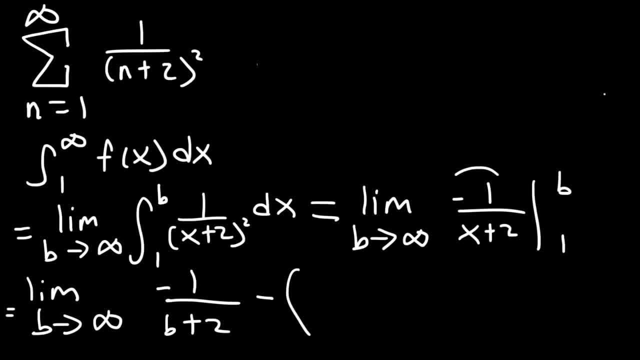 2, and then minus. now we need to plug in 1, so it's going to be negative 1 over 1 plus 2, which is 3.. Now the limit as b approaches infinity for negative 1 over b plus 2, that's. 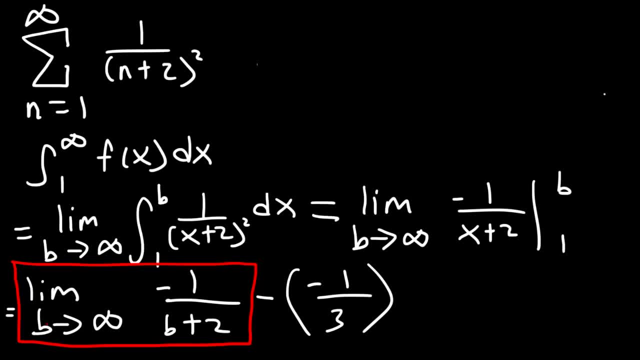 going to go to 0. If it was 1 over b, that would go to 0 as well. so negative 1 over b plus 2, that's also going to go to 0.. And then we have minus negative 1. third, so this: 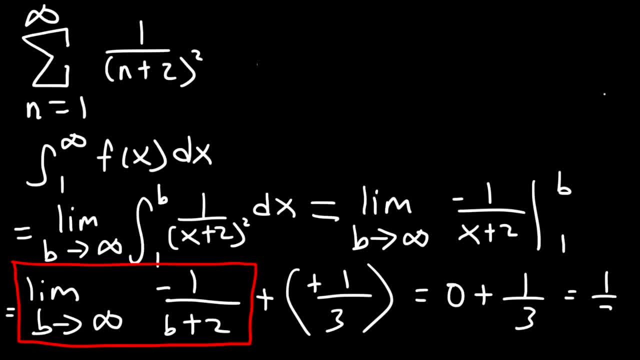 is going to be plus 1 third. So because we get a finite value, we could say that the integral converges to 1 over 3.. So if the integral converges, then according to the integral test, the series must also. 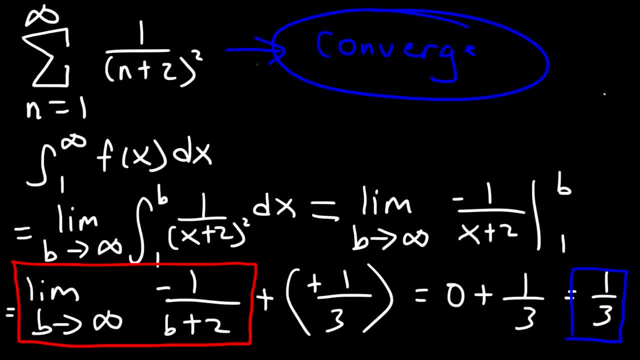 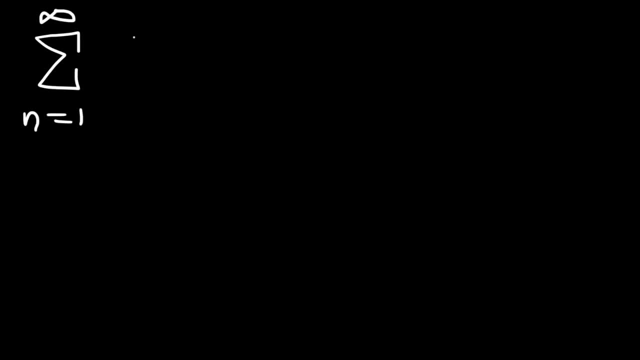 converge. And so that's it for this problem. Now let's try another example. So let's say we have a series with the sequence 2n over 3n, squared plus 4.. So go ahead and use the integral test to determine if the series will converge or diverge. So let's begin by writing. 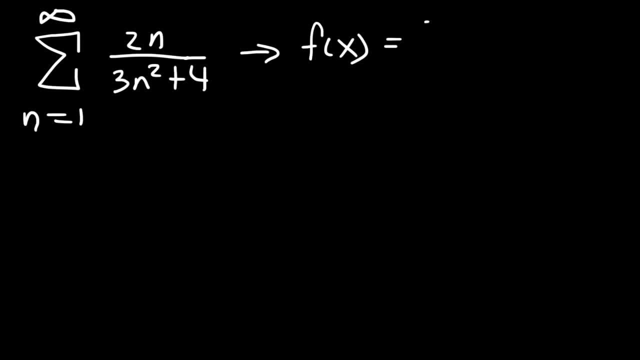 the corresponding function: 2x divided by 3x squared plus 4.. Now there are no points of discontinuity for this function. So the function is definitely continuous. Is it positive? Well, when x is greater than or equal to 1, it will always be positive. 2x will be positive when x is a positive number. 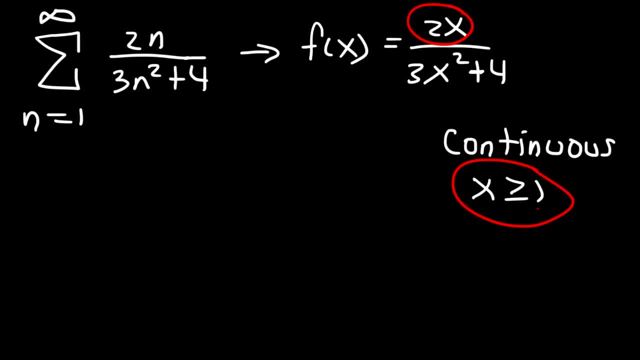 It will only be negative when x is a positive number. It will only be negative when x is a positive number. It will only be negative when x is less than 0. And since x is equal to or greater than 1,, 2x will be positive And 3x squared plus 4, that's going to be positive as well, Because 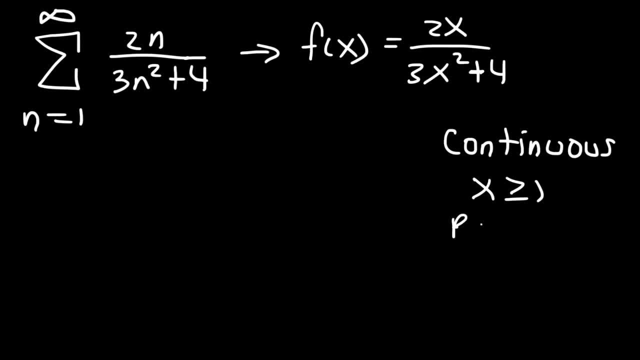 x squared is always positive, So we have a positive function. Now is it a decreasing function? So we need to find the first derivative in order to determine that. Now we're going to have to use the quotient rule to get the answer. 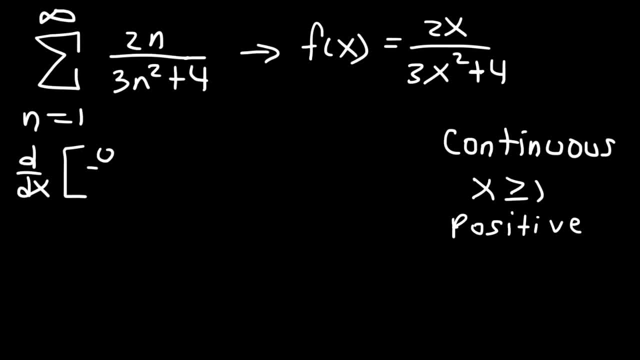 So, if you recall, the derivative of u over v is going to be vu prime minus uv prime over v squared. So u in this example is 2x, v is 3x squared plus 4.. So f prime of x is going. 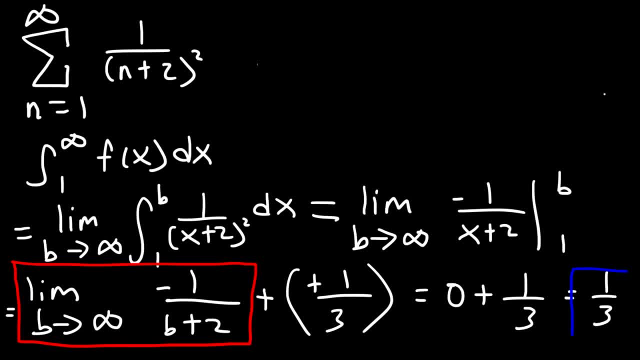 So because we get a finite value, we can say that the integral converges to 1 over 3.. So if the integral converges, then according to the integral test, the series must also converge. And so that's it for this problem. 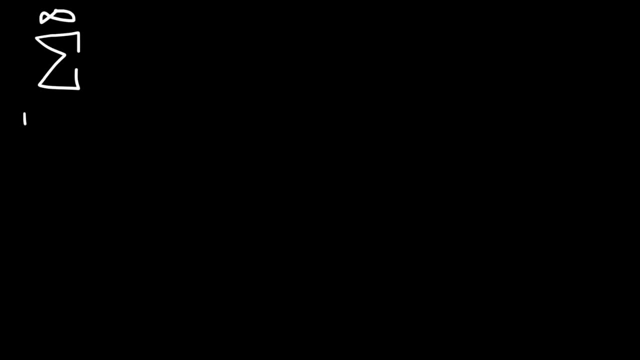 Now let's try another example. So let's say we have a series with the sequence 2n over 3n, squared plus 4.. So go ahead and use the integral test to determine if the series will converge or diverge. So let's begin by writing the corresponding function. 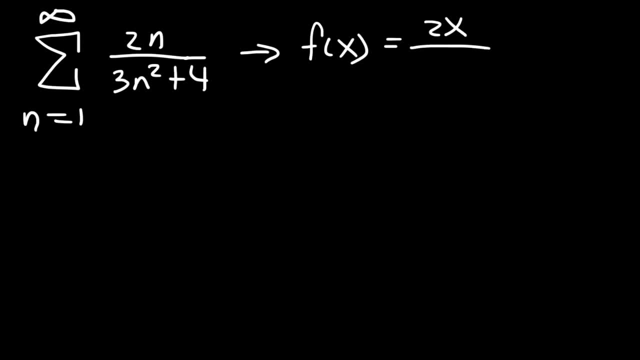 So f of x is going to be 2x divided by 2. That's going to be 4x squared plus 4.. So if f of x is going to be 2x, that's going to be the series wins. 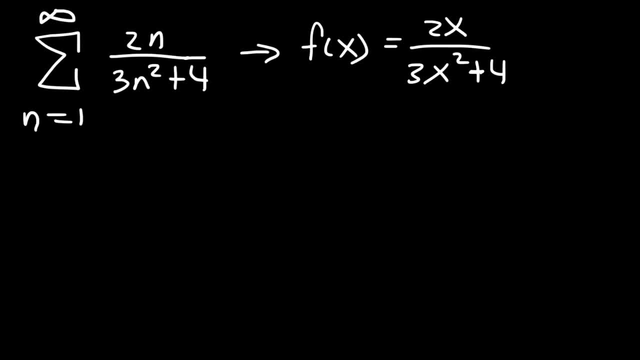 Now, there are no points of discontinuity for this function, so the function is definitely continuous. Is it positive? Well, when x is greater than or equal to 1, it will always be positive. 2x will be positive when x is a positive number. 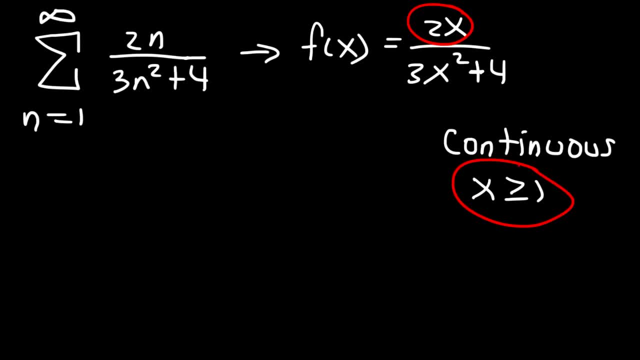 It will only be negative when x is less than 3.. 0. And since x is equal to a greater than 1,, 2x will be positive And 3x squared plus 4, that's going to be positive as well, because x squared is always positive. 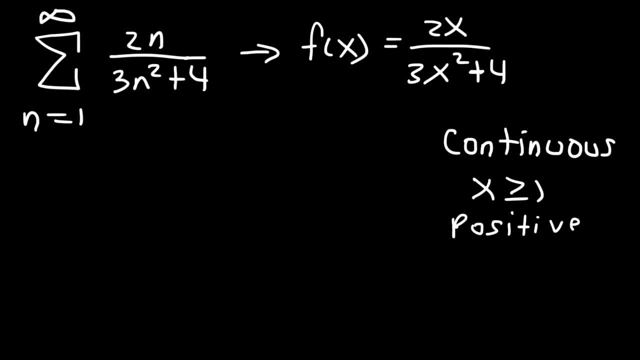 So we have a positive function. Now is it a decrease in function? So we need to find the first derivative in order to determine that. Now we're going to have to use the quotient rule to get the answer. So, if you recall, the derivative of u over v is going to be vu, prime minus uv, prime over v squared. 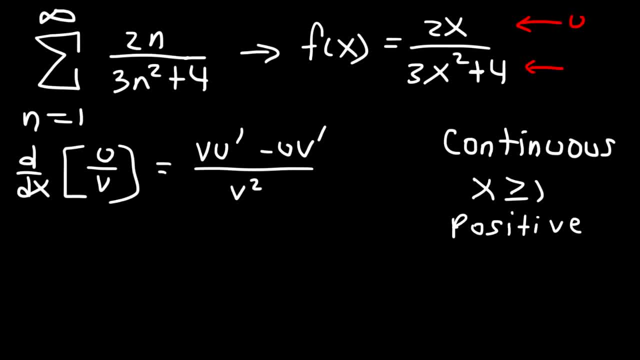 So u in this example is 2x, v is 3x squared plus 4.. So f prime of x is going to be v, which is this times u prime. so that's 2, minus u, and then times v prime, which is 2.. 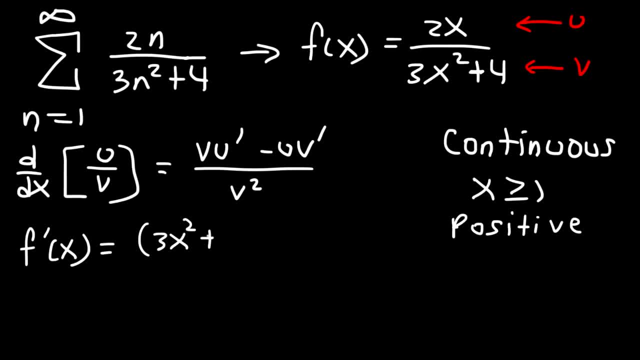 to be v, which is this times u prime, so that's 2, minus u, and then times v prime, which is 6x All divided by v squared, And that's 3x squared plus 4 squared. 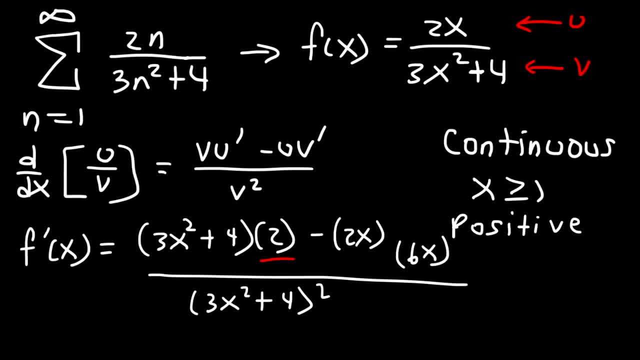 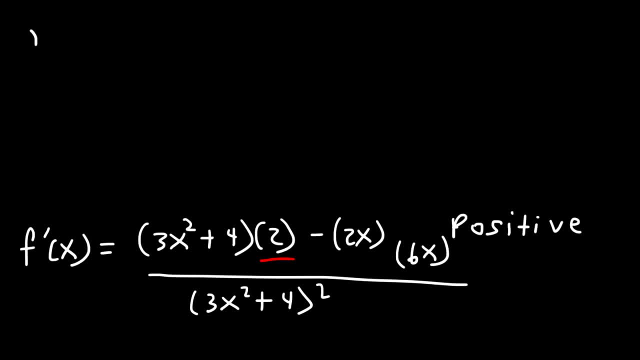 So let's begin by distributing the two. So first I'm just going to have to get rid of some stuff, And so this is going to be 6x squared plus 8. And then 2x times 6x, that's 12x. And then 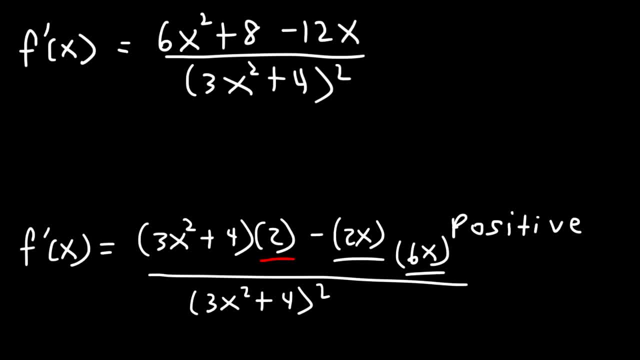 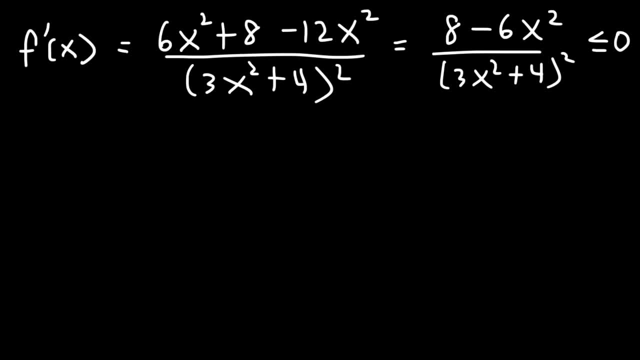 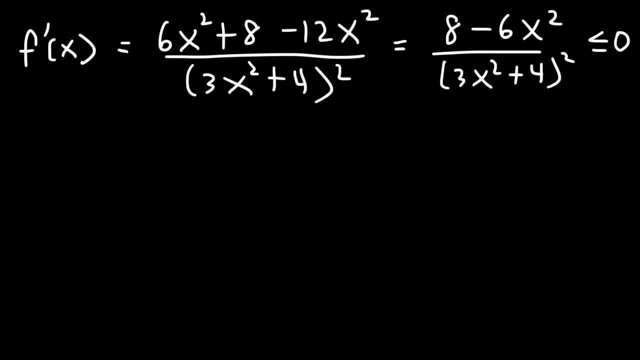 3x squared plus 4 will never be 0.. Now we can set the numerator equal to 0.. If we add 6x squared to both sides, we'll get this, And then we'll divide by 6. 0.. 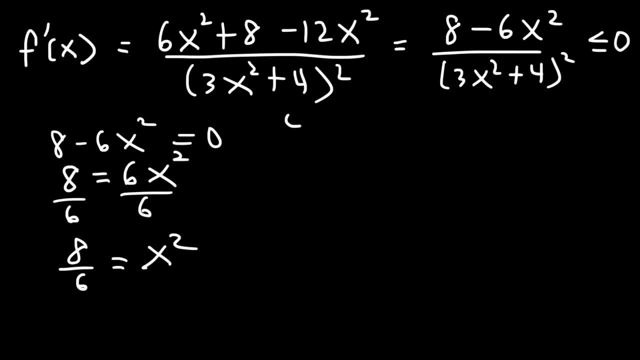 So 8 over 6 is equal to x squared, and then we can reduce that to 4 over 3.. So, taking the square root of both sides, we're going to get plus or minus 2 over the square root of 3.. 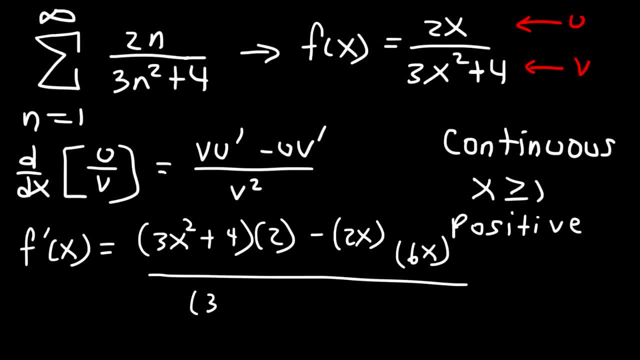 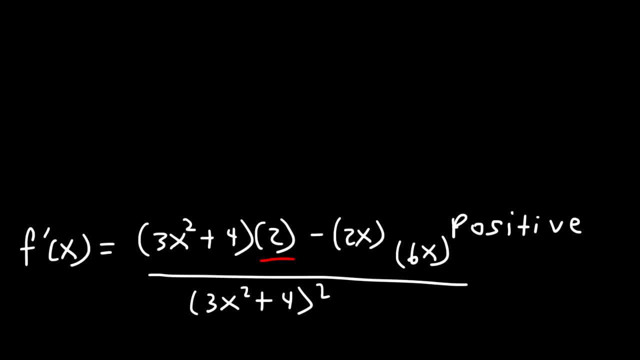 So that's 6x all divided by v squared, and that's 3x squared plus 4 squared. So let's begin by distributing the two. So first I'm just going to have to get rid of some stuff, And so this is going to be 6x squared plus 8, and then 2x times 6x, that's 12x. 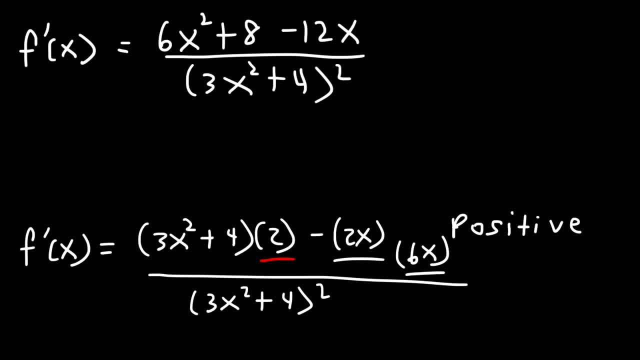 And then 6, this should be 12x squared. 6x squared minus 12x squared, that's going to be negative 6x squared. Now let's see when this expression is less than or equal to 0.. We want to determine when it's negative. 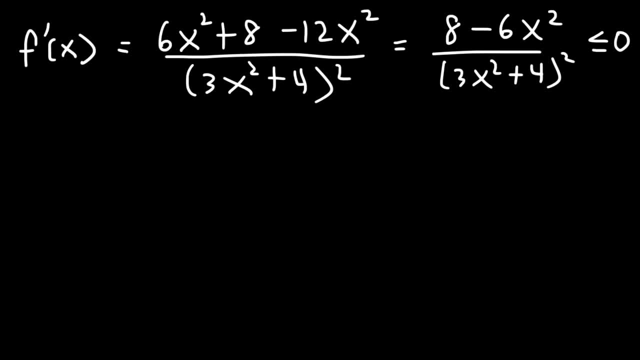 So let's identify the critical points. If we set the denominator equal to 0, we're not going to get any values, for x, 3x squared plus 4 will never be 0.. Now we can set the numerator equal to 0.. 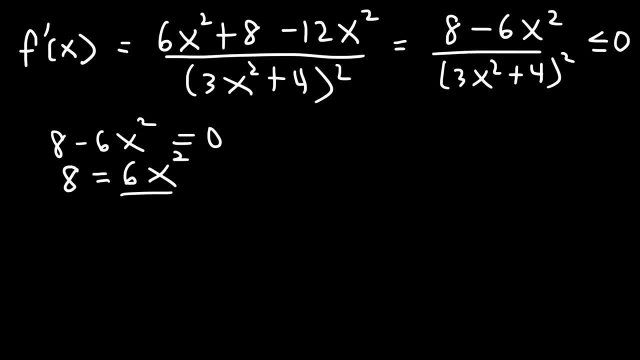 If we add 6x squared to both sides, we'll get this and then we'll divide by 6.. So 8 over 6 is equal to x squared, and then we can reduce that to 4 over 3.. So, taking the square root of both sides, we're going to get plus or minus 2 over the square root of 3.. 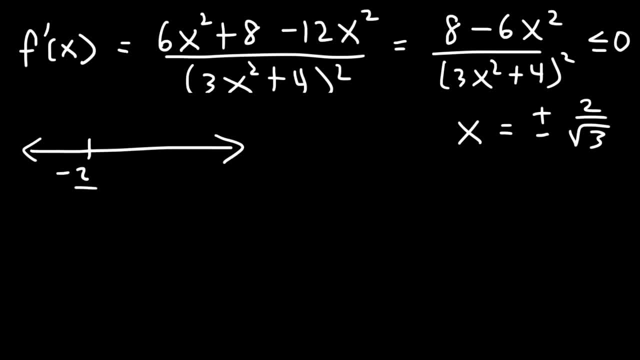 Now let's create a sine chart. Now: 2 divided by the square root of 2.. 2 divided by the square root of 3, as a decimal, that's 1.155 approximately. So we need it to be negative from 1 to infinity. 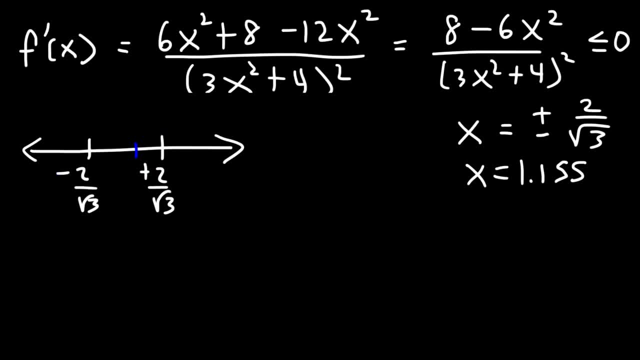 So 1 is somewhere in this region. Just keep that in mind. Now let's say, if we plug in 2.. 8 minus 6 times 2 squared, Is that going to be positive or negative? If you plug in 2, this will be negative, but on the bottom that's always going to be positive. 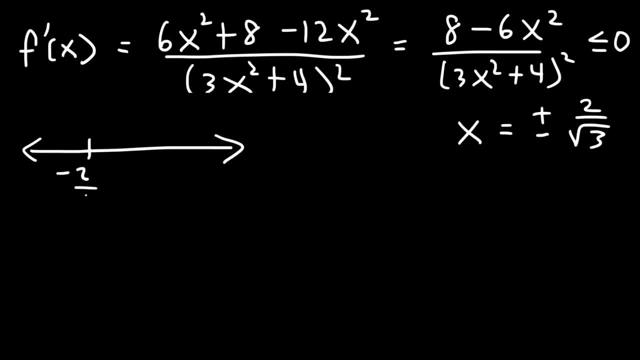 Now let's create a sine chart. Now: 2 divided by the square root of 3, as a decimal that's 1.155, approximately. So we need it to be negative from 1 to infinity. So 1 is somewhere in this region. 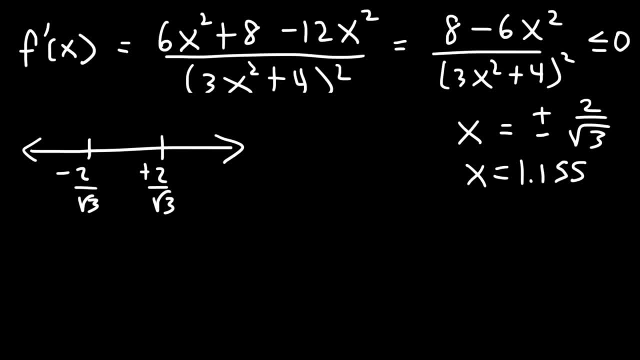 Just keep that in mind. Now let's say, if we plug in 2.. 8 minus 6 times 2 squared, Is that going to be positive or negative? If you plug in 2, this will be negative, but on the bottom that's always going to be positive. 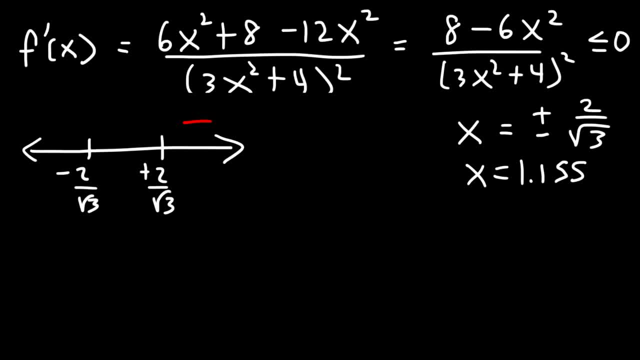 So this is negative in this region. Now, if we plug in 0, 8 minus 6 times 0, squared, that's 8. And that's negative, And that's negative, And the bottom will still be positive. 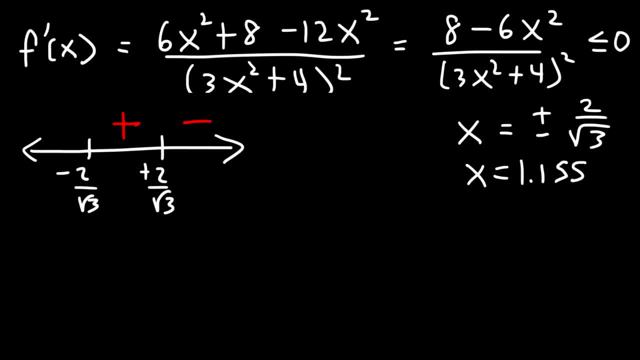 So therefore, this will be positive in this region And then if we plug in, let's say, negative 4, the numerator will be negative And the bottom will be positive. so this is going to be negative. So, looking at the sine chart, we know the function is decreasing from 2 over square root, 3 to infinity. 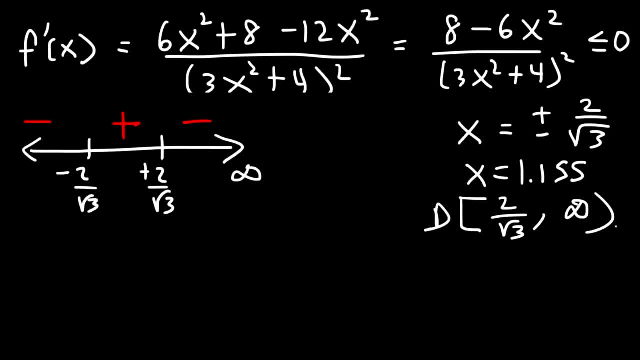 But it's not decreasing from 1 to infinity, so we can't use the integral test In that region. We could, however, use the integral test from 2 to infinity because it's continuous there, And we can't use this number in a sequence because it's not an integer. 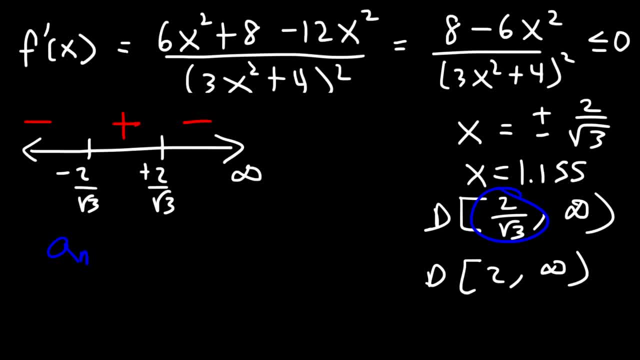 For the sequence a, sub n, you can only use integers. So let's determine the integral from 2 to infinity and let's see if it converges or diverges. So f of x is 2x over 3x squared plus 4.. 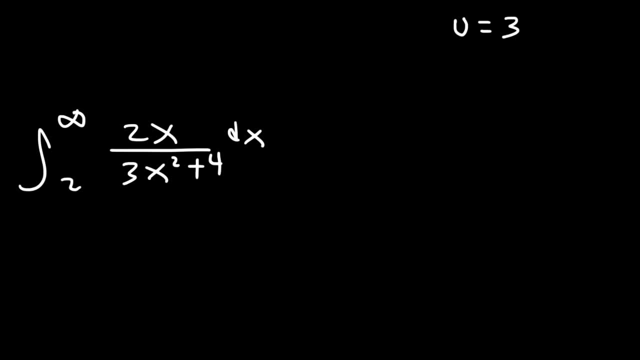 So let's use u substitution. We're going to make u equal to 3x squared plus 4.. And so du is going to be 6x dx, And so dx is du over 6x. So this is going to be u on the bottom, and then replace dx with du over 6x. 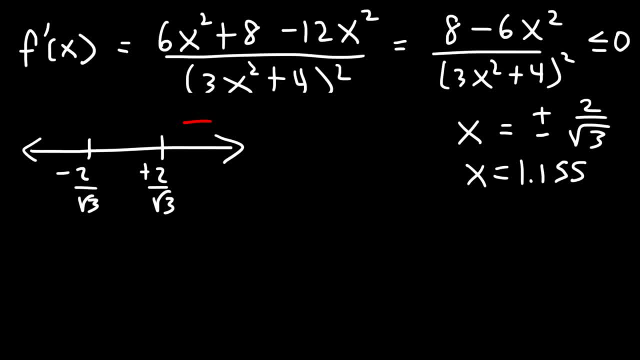 So this is negative in this region. Now, if we plug in 0, 8 minus 6 times 0, squared, that's 8. And the bottom will still be positive. So therefore, this will be positive in this region. And then if we plug in, let's say, negative, 4.. 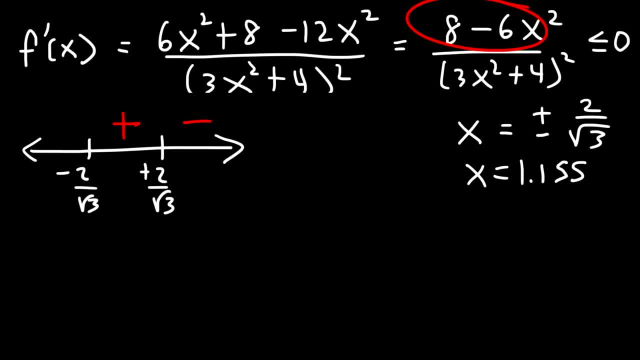 The numerator will be negative and the bottom will be positive, so this is going to be negative. So, looking at the sine chart, we know the function is decreasing from 2 over square root, 3 to infinity, But it's not decreasing from 1 to infinity, so we can't use the integral test in that region. 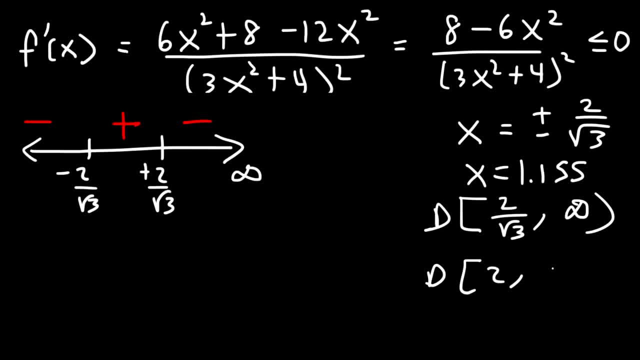 We could, however, use the integral test from 2 to infinity, because it's continuous there, And We can't use this number in a sequence because it's not an integer, For the sequence, a sub n. you can only use integers. 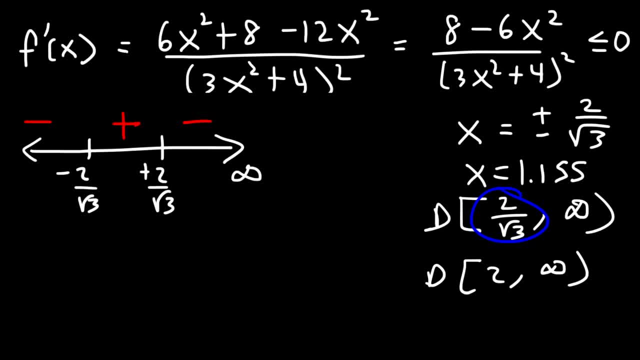 So let's determine the integral from 2 to infinity and let's see if it converges or diverges. So f of x is 2x over 3x squared plus 4.. So f of x is 2x over 3x squared plus 4.. 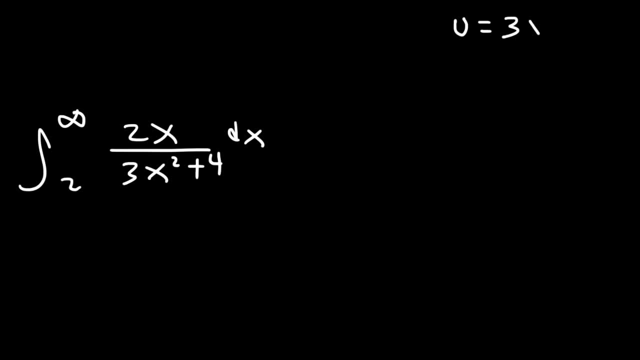 So let's use u-substitution. We're going to make u equal to 3x squared plus 4.. And so du is going to be 6x dx, And so dx is du over 6x. So this is going to be u on the bottom, and then replace dx with du over 6x. 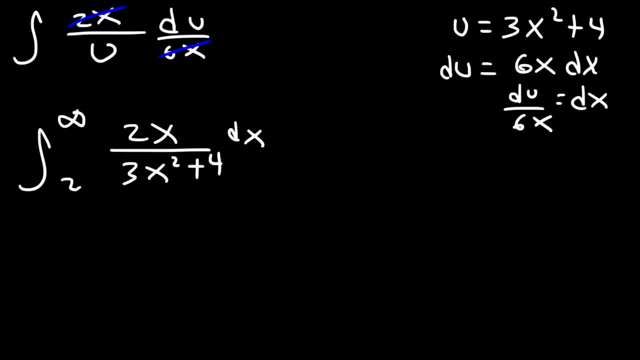 So 2x over 6x, that's going to be 1- 3rd. So this is 1 3rd times the integral of 1 du, which is going to be 1 3rd ln u, And then that's going to be 1 3rd ln. 3x squared plus 4.. 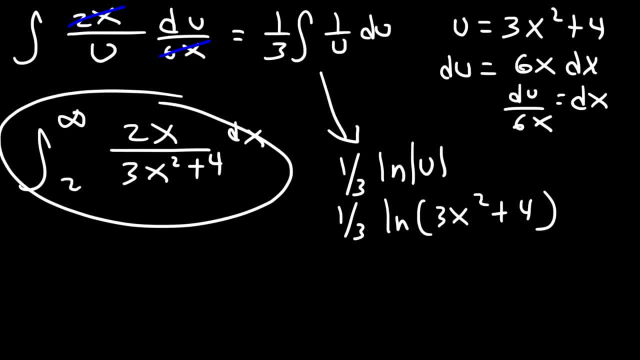 So now we're going to make this integral equal to the limit As b approaches infinity for the integral 2 to b, 2x over 3x squared plus 4 dx, And so that's going to be the limit as b approaches infinity. 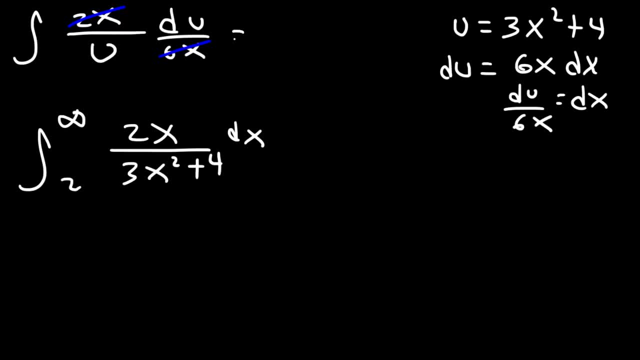 So 2x over 6x, that's going to be 1 third. So this is 1 third times the integral of 1 du, which is going to be 1 third ln u, And then that's going to be 1 third ln 3x squared plus 4.. 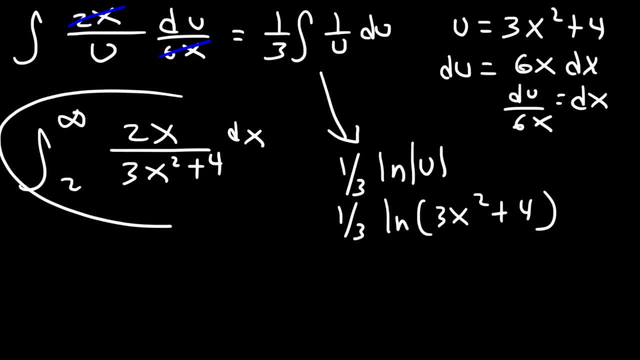 So now we're going to make this integral equal to the limit as b approaches infinity, for the integral 2 to be 2x over 3x squared plus 4 dx, And so that's going to be the limit as b approaches infinity. 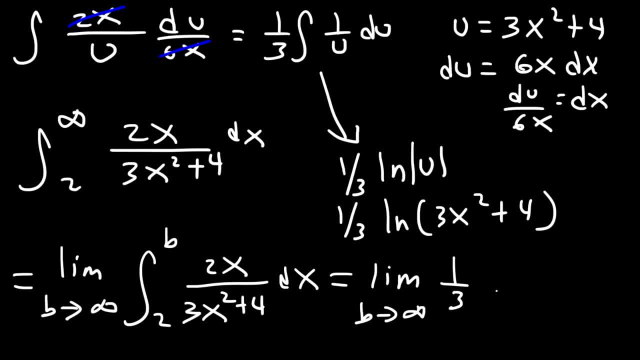 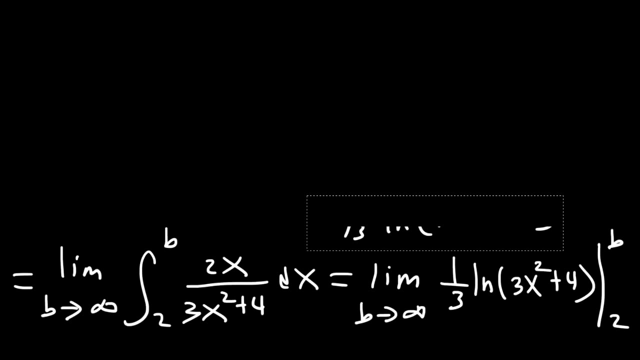 And so we're going to get 1 third ln, 3x squared plus 4. Evaluated from 2 to b. So we no longer need the absolute value expression because 3x squared plus 4 is always positive. So we now have the limit as b approaches infinity. 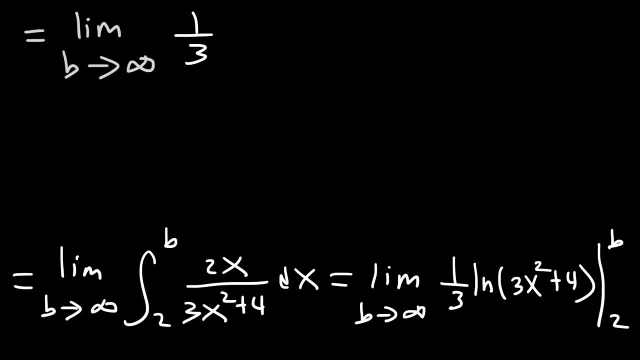 And then this is 1 third ln. 3x squared plus 4 dx. We're going toさp the first core 취 3b squared plus 4, and then minus. Now let's plug in 2.. So 1 third ln 2 squared is 4 times 3, that's. 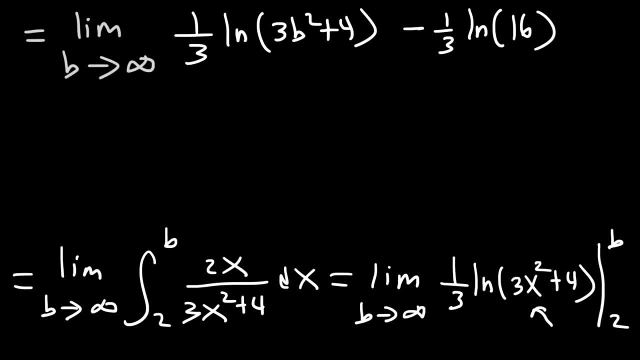 12 plus 4, that's 16.. Now, as b goes into infinity, what happens to ln. 3b squared plus 4? infinity squared is infinity. if you multiply that by 3, then add 4, you're still going to get infinity, and the natural log of infinity is still. 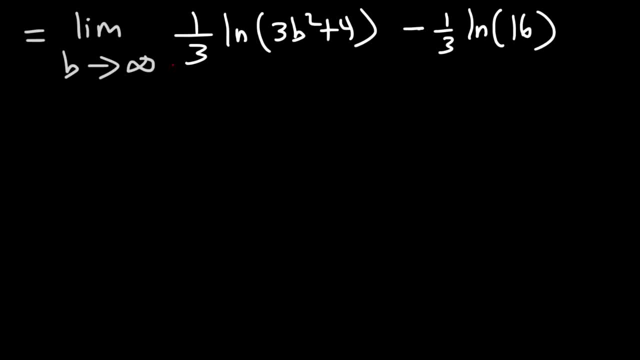 infinity. So this entire expression goes to infinity. So infinity minus some finite number is still going to be infinity. Therefore, since the integral from 2 to infinity of f, of x, dx, because it equals infinity, it doesn't equal a finite number, we could say that the integral diverges. and if the integral diverges, then the series. 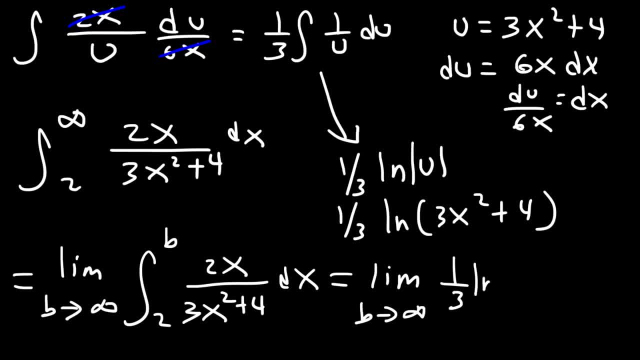 And so we're going to get 1, 3rd ln, 3x squared plus 4, evaluated from 2 to b. So we no longer need the absolute value expression, because 3x squared plus 4, is always positive. 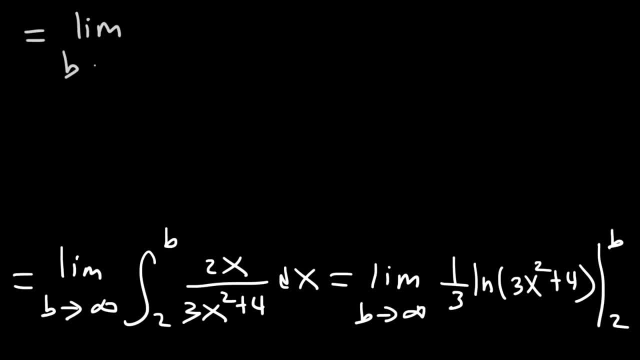 So we now have the limit as b approaches infinity. And then this is 1, 3rd natural log: 3 b squared plus 4, and then minus. Now let's plug in 2.. So 1, 3rd ln. 2 squared is 4, times 3, that's 12 plus 4,, that's 16.. 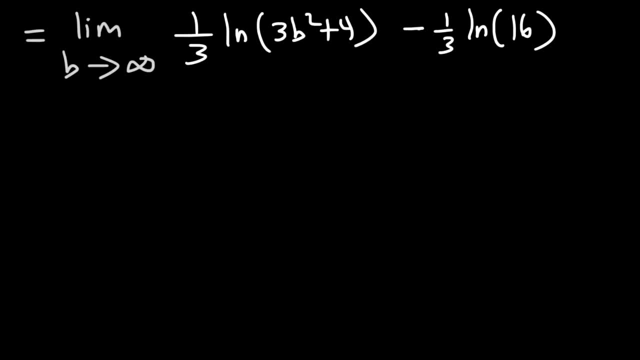 Now, as b goes into infinity, what happens to ln 3, b squared plus 4? Infinity squared is infinity. If you multiply that by 3, then add 4, you're still going to get infinity, And the natural log of infinity is still infinity. 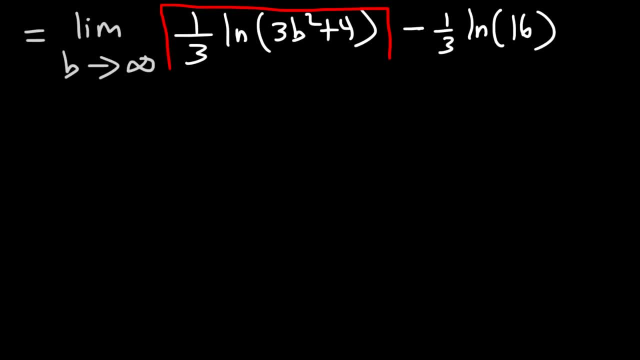 So this, this entire expression goes to infinity. So infinity minus some finite number is still going to be infinity. Therefore, since the integral from 2 to infinity of f, of x, dx, because it equals infinity, it doesn't equal a finite number. 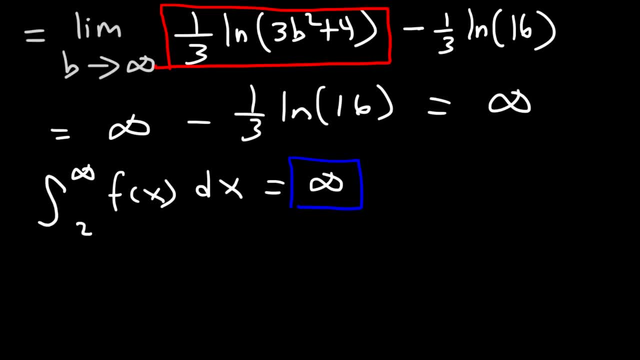 we could say that the integral diverges. And if the integral diverges, then the series from 2 to infinity of a sub n, which was 2n over 3n squared plus 4, this will also diverge. Now, if this series diverges, what about the original series? 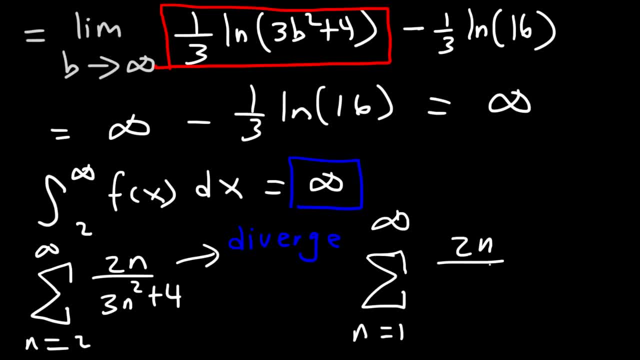 Let's say from 1 to infinity. The only difference between these two series is that this one has an extra term, the a sub 1 term. So if we add the second term to an infinite number of terms and we get a divergent sum, 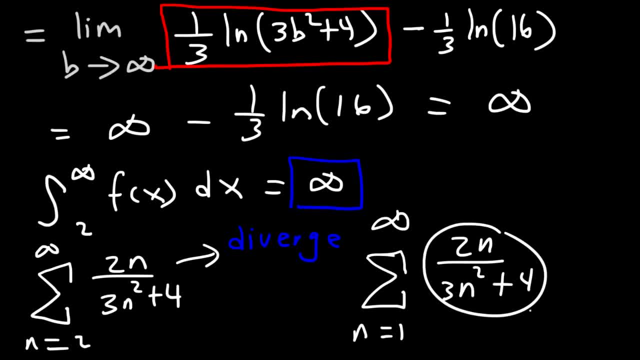 then if we add the first term to basically a divergent sum of infinity, the first term plus infinity will still be equal to infinity. So therefore this series must also diverge, And so that's the answer for this problem. We have a divergent series. 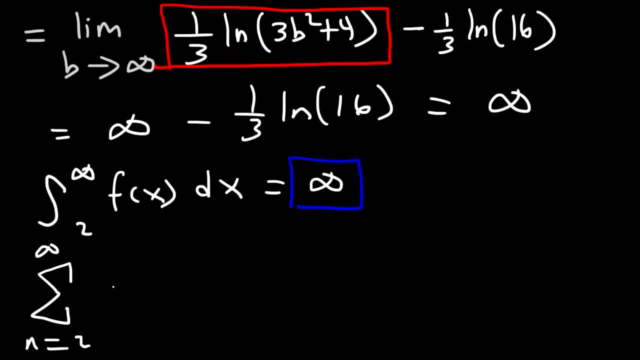 from 2 to infinity, of a sub n which was 2n over 3n squared plus 4. this will also diverge. Now, if this series diverges, what about the original series? let's say from 1 to infinity, The only difference. 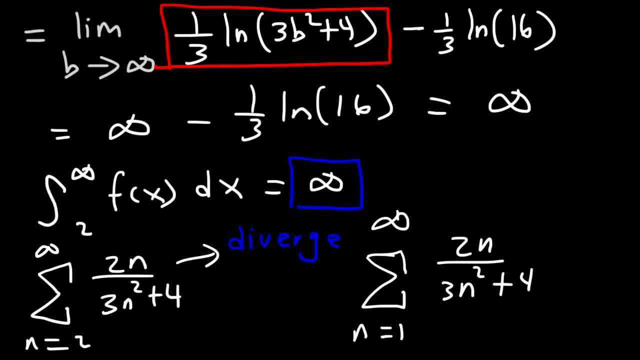 between these two series is that this one has an extra term, the, a sub 1 term. So if we add the second term to an infinite number of terms and we get a divergent sum, then if we add the first term to basically a divergent sum of infinity, the first term plus infinity will still be equal. 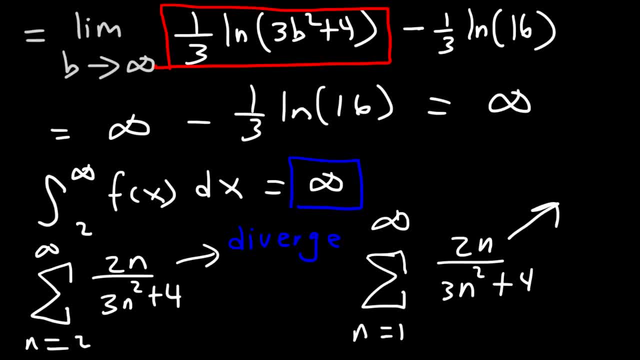 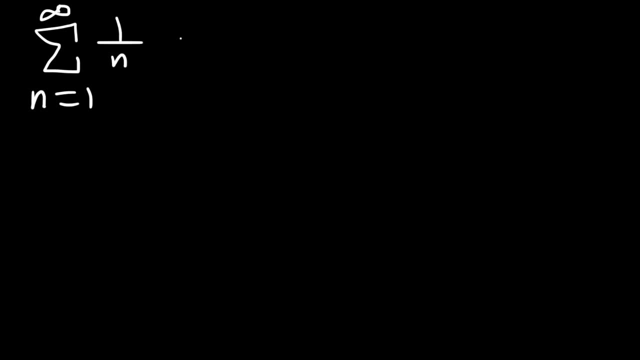 to infinity. So therefore, this series must also diverge, And so that's the answer for this problem. We have a divergent series. Now let's talk about the harmonic series from 1 to infinity. If we list out the terms, it's going to be 1 plus 1 half plus 1 over 3. 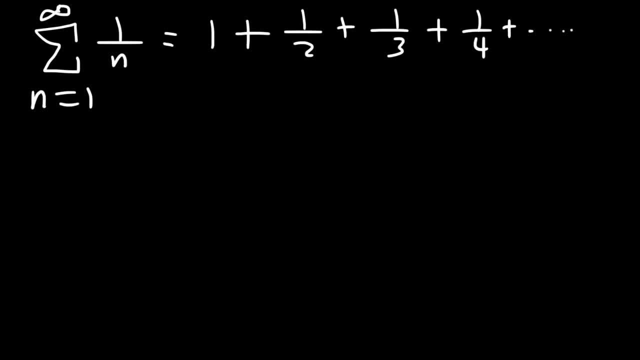 plus 1 over 4. and so forth. Now we know that the harmonic series is the divergent series, but use the integral test to show that it's divergent. So let's begin with the corresponding function, 1 over x, and let's draw a graph of it. Now the graph: 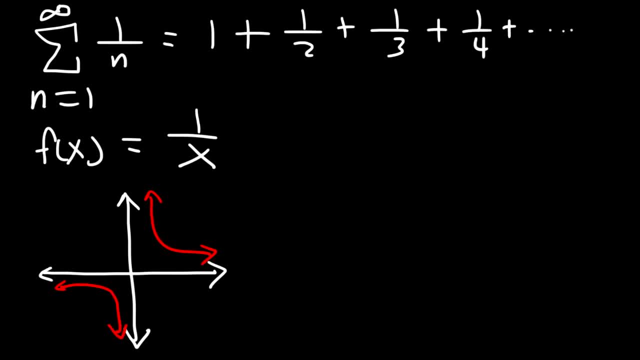 looks like this and it has a vertical asymptote at x equals 0, but let's focus from 1 to infinity. So, from 1 to infinity, the function is positive because it's above the x-axis. It's also continuous from 1 to infinity. There's no infinite. 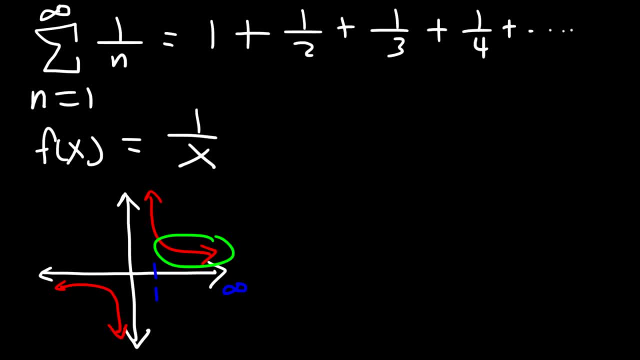 discontinuities, no holes, no jump discontinuities in that region. And finally, you can see that it's decreasing from 1 to infinity. It's going down. So all three conditions are met for this particular function. So we could use the. 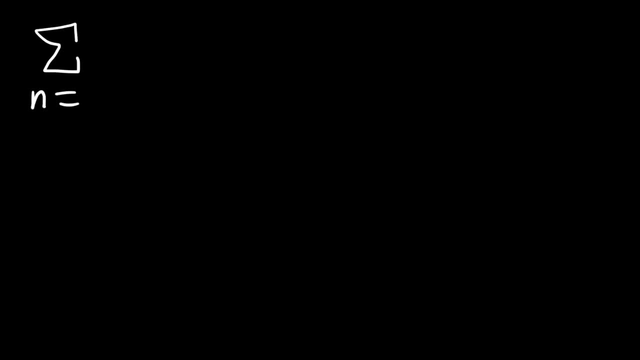 Now let's talk about the harmonic series from 1 to infinity. If we list out the terms, it's going to be 1 plus 1 half, plus 1 over 3, plus 1 over 4, and so forth. 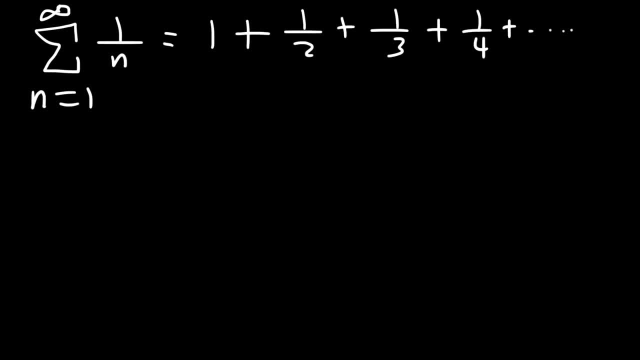 Now we know that the harmonic series is the divergent series, but use the integral test to show that it's divergent. So let's begin with the corresponding function: 1 over x. Now let's draw a graph of it. 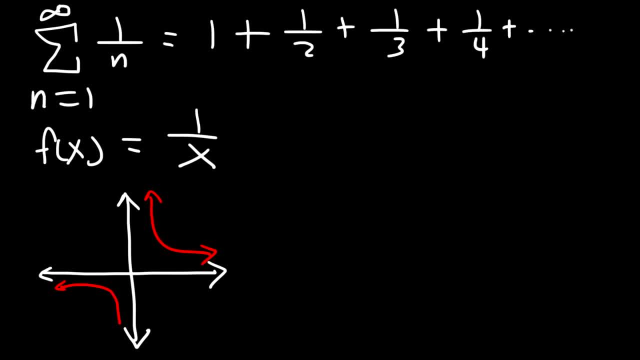 Now the graph looks like this and it has a vertical asymptote at x equals 0.. But let's focus from 1 to infinity. So from 1 to infinity, the function is positive because it's above the x axis. It's also continuous from 1 to infinity. 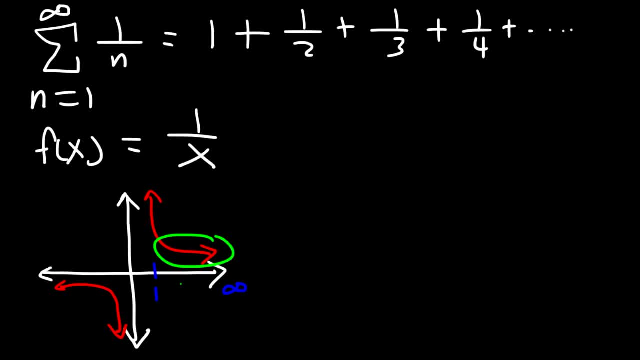 There's no infinite discontinuities, no holes, no jump discontinuities in that region And finally, you can see that it's decreasing from 1 to infinity. It's going down. So all three conditions are met for this particular function. 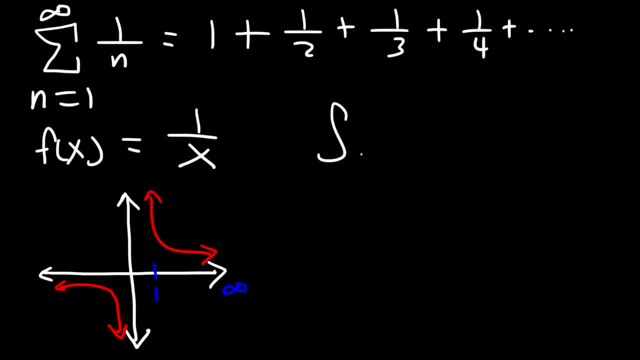 So we could use the integral test. So let's integrate it from 1 to infinity: 1 over x, dx. So this is going to equal the limit as b approaches infinity. integral 1 to b: 1 over x, dx. The antiderivative of 1 over x is the natural log of x. 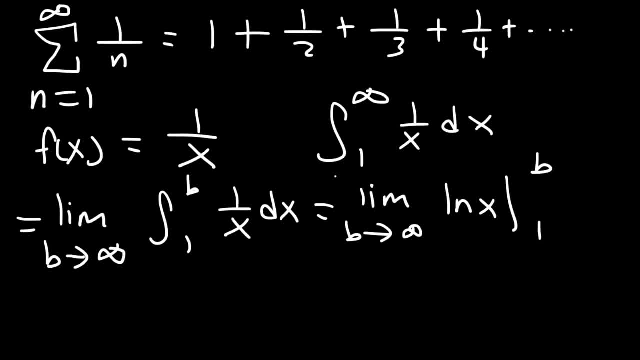 And let's evaluate from 1 to b, as b goes to infinity. So we're going to have the limit as b goes to infinity: ln b minus ln 1.. Now the natural log of infinity is infinity and ln 1 is 0.. 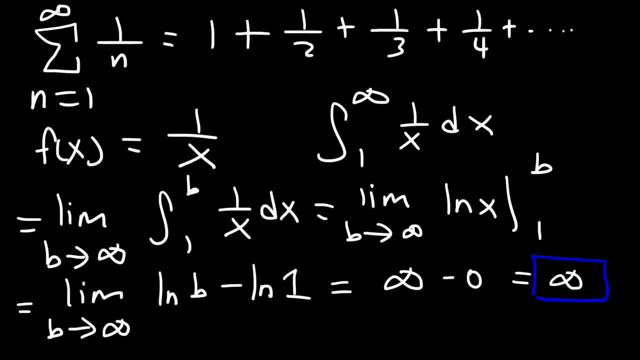 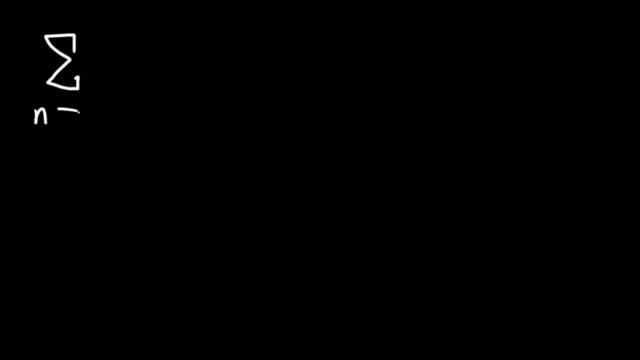 So, therefore, the integral diverges to infinity, which means that the series also diverges. Now let's talk about this particular series. Let's say it's 2 divided by n squared plus 6n plus 10.. So go ahead and use the integral test. 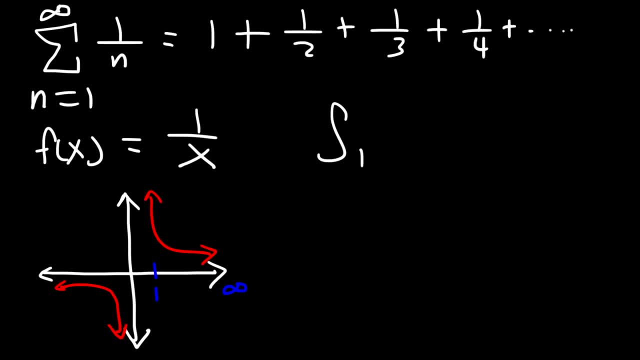 integral test. So let's integrate it from 1 to infinity: 1 over x, dx. So this is going to equal the limit as b approaches infinity. integral 1 to b: 1 over x, dx. The antiderivative of 1 over x is the natural log of x. And let's evaluate from 1 to b. 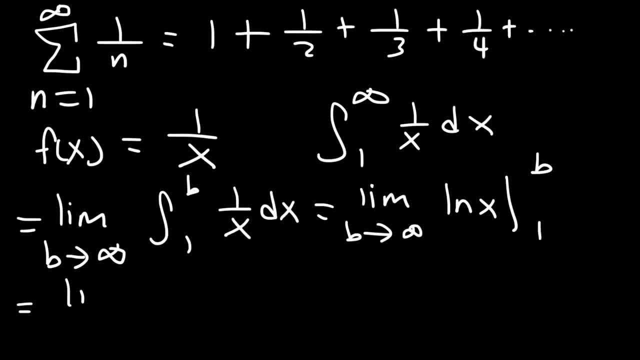 as b approaches infinity. So we're going to have the limit as b goes to infinity: ln b minus ln 1.. Now the natural log of infinity is infinity and ln 1 is 0. So therefore the integral diverges to infinity, which means that the series also diverges. Now 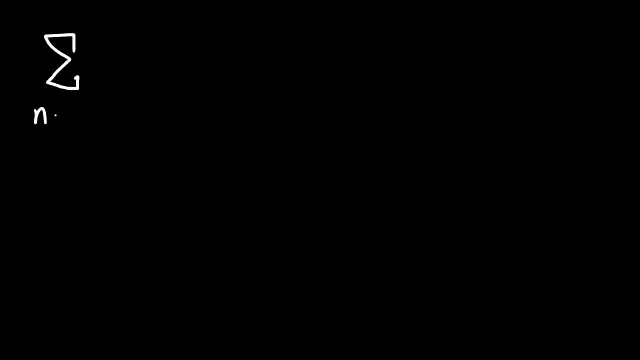 let's talk about this particular series. Let's say it's 2 divided by n squared plus 6n plus 10.. So go ahead and use the integral test to see if the series is going to converge or diverge. Now the first thing I would recommend doing is rearranging this expression. So 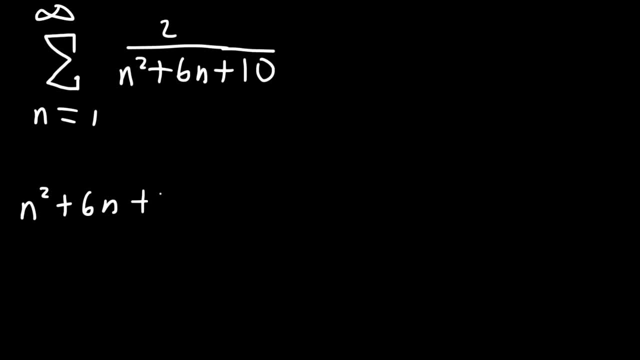 let's focus on n squared plus 6n. Now let's complete the square. So half of 6 is 3, and 3 squared is 9.. So instead of writing 10,, I'm going to write 9 plus 1,, because this is a perfect square trinomial. 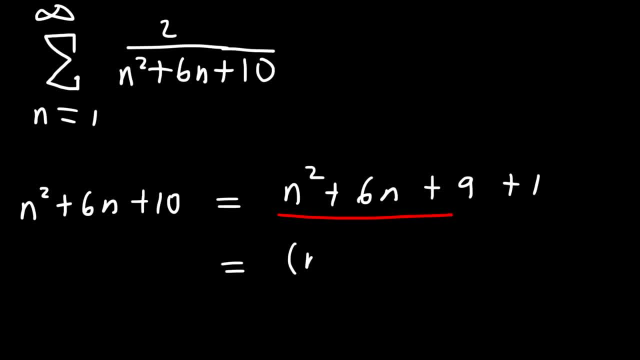 Two numbers that multiply to 9 but add to 6 is 3.. So it's going to be n plus 3 times n plus 3, which we can write as n plus 3 squared plus 1.. So we're going to write n plus 3 times n plus 3, which we can write as n plus 3 squared. 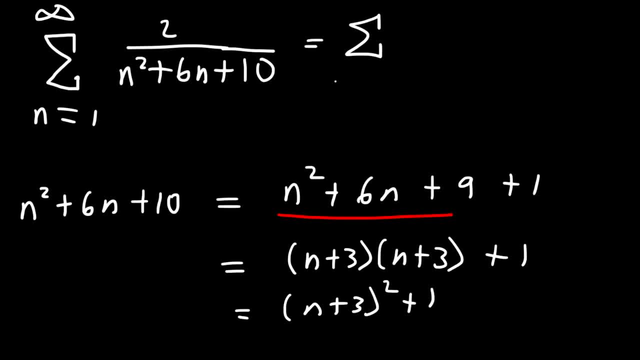 plus 1.. So now we have this particular series. So now let's write the corresponding function. So f of x is going to be 2 divided by x plus 3 squared plus 1.. So is this function always positive? Yes, it is always positive. 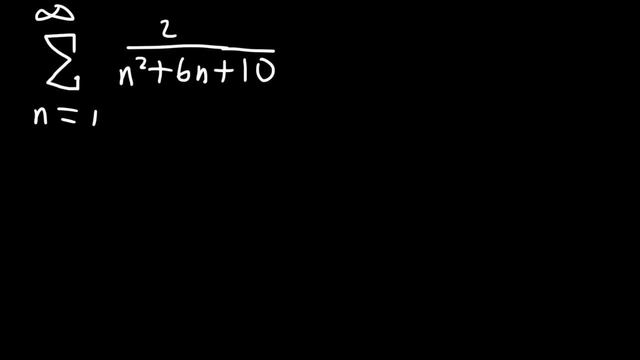 to see if the series is going to converge or diverge. Now the first thing I would recommend doing is rearranging this expression. So let's focus on n squared plus 6n plus 10.. And let's complete the square. So half of 6 is 3, and 3 squared is 9.. 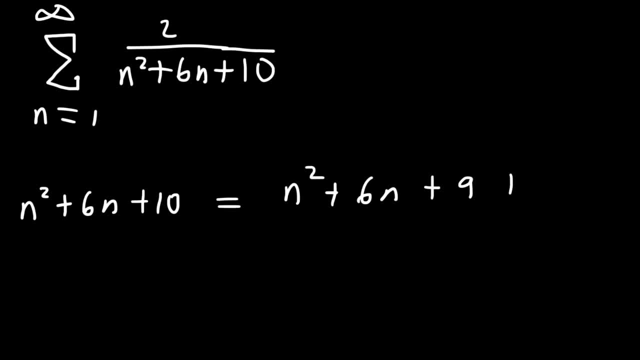 So instead of writing 10,, I'm going to write 9 plus 1.. Because this is a perfect square trinomial: Two numbers that multiply to 9, but add to 6 is 3.. So it's going to be n plus 3 times n plus 3,. 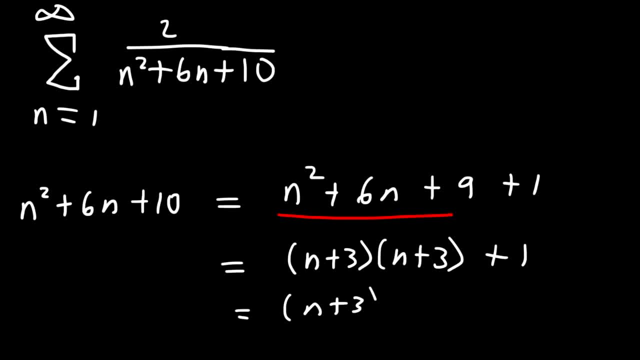 which we can write as n plus 3 squared plus 1.. So now we have this particular series. So now let's write the corresponding function. So f of x is going to be 2 divided by x plus 3, squared plus 1.. 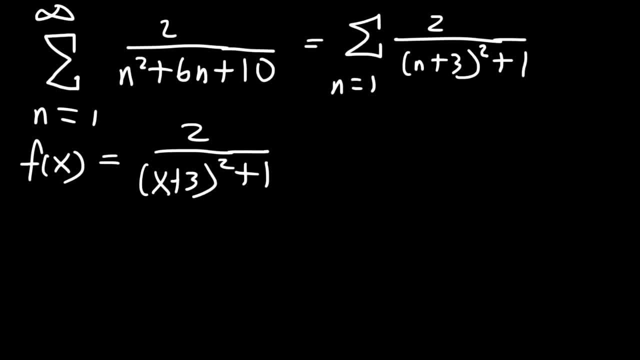 So is this function always positive? x plus 3 squared will always be positive and everything else is positive, So this function is always going to be positive everywhere. Now is it continuous? There are no points of discontinuity. x plus 3 squared is always positive. 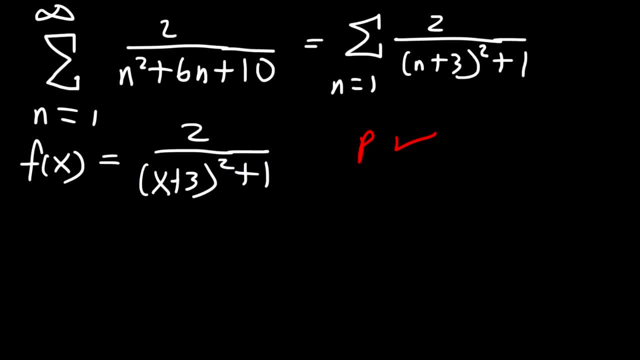 and then if you add 1 to it, it will never be 0 on the bottom, So it's continuous everywhere. There are no points of discontinuity. Now is it a decreasing function? The fact that it's a bottom-heavy function? that's always positive. 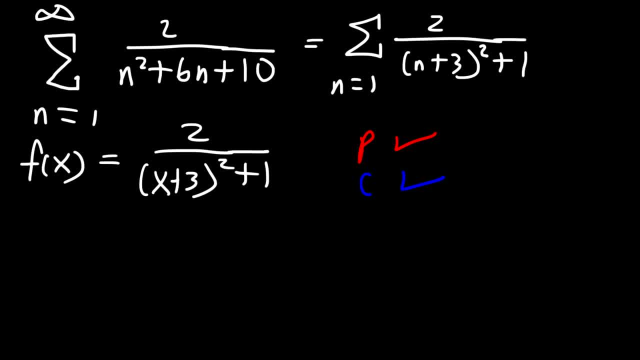 indicates that it's a decreasing function. But if you want to, you can go ahead and find the first derivative. If you were to draw a rough sketch of the graph of this function, you'll see that at negative 3, it has its highest value of 2.. 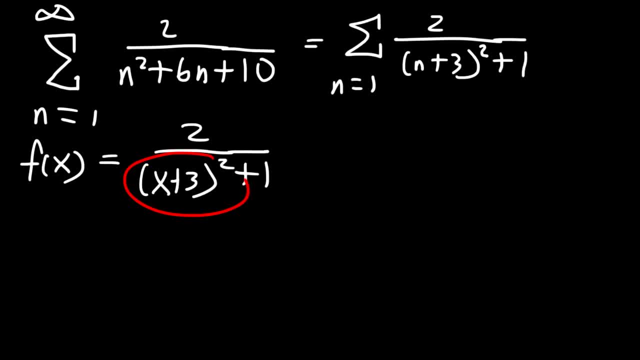 Okay, so now let's write the corresponding function. So f of x is going to be 2 divided by x plus 3 squared plus 1.. So is this function always positive? Yes, it is always positive. x plus 3 squared will always be positive and everything else is positive. 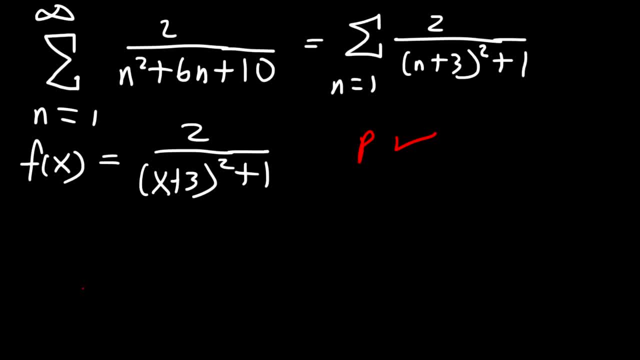 So this function is always going to be positive everywhere. Now is it continuous? There are no points of discontinuity. x plus 3 squared is always positive, and then if you add 1 to it, it will never be zero on the bottom. 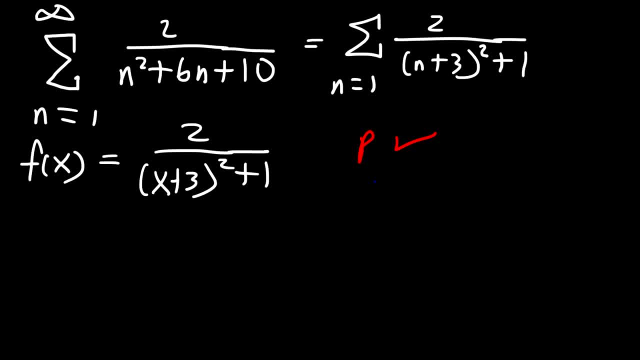 So it's continuous everywhere. There are no points of discontinuity. Now, is it a decrease in function? The fact that it's a bottom-heavy function- that's always positive- indicates that it's a decreasing function. But if you want to, you can go ahead and find the first derivative. 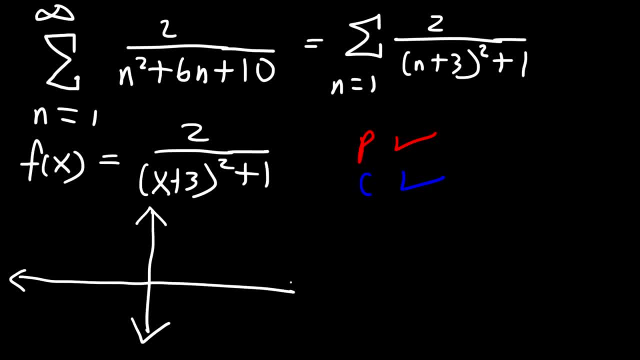 If you were to draw a rough sketch of the graph of this function, you'll see that at negative 3, it has its highest value of 2.. Negative 3 plus 3,, that's 0, and so it becomes 2 over 1.. 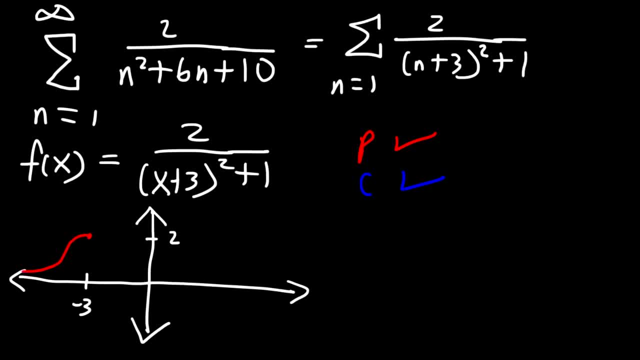 And so that's the maximum value of the function, And then, after that point, it follows the x-axis. And so if we focus on a region from 1 to infinity, you can see that it's a decreasing function, it's positive, it's above the x-axis and it's continuous everywhere, from 1 to infinity. 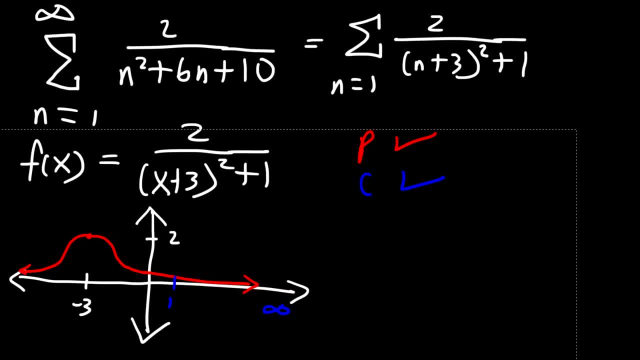 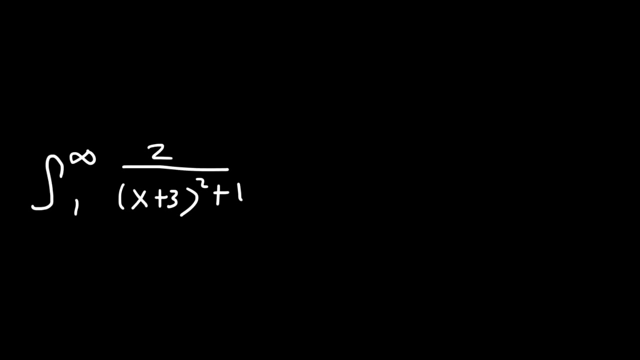 So we can use the integral test for that function. Now let's find the integral from 1 to infinity of the corresponding function: 2 over x plus 3 squared plus 1.. So for this problem we need to use trig substitution. 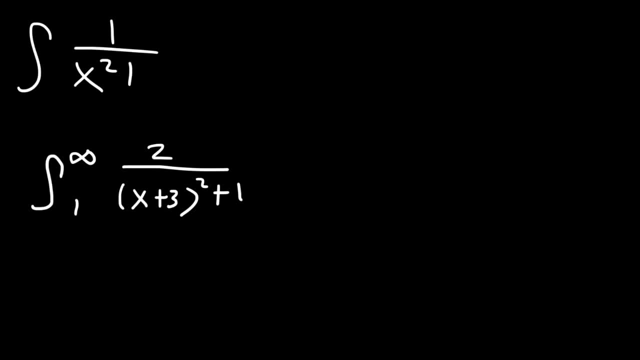 And if you see an integral with this generic formula or a generic expression, this is equal to arctangent of x. So this is going to be equal to something related to arctangent. So what we're going to do is replace x plus 3 with tangent theta. 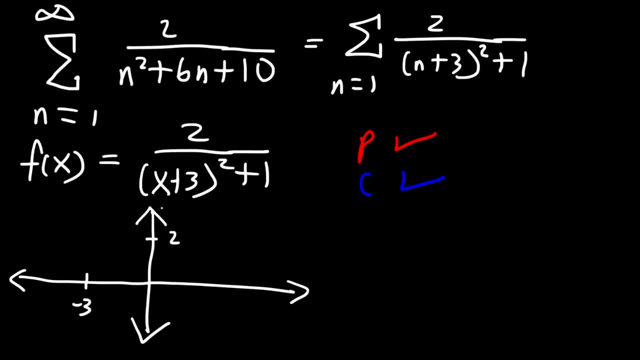 Negative, 3 plus 3, that's 0.. And so it becomes 2 over 1.. And so that's the maximum value of the function. And then, after that point it just it follows the x-axis. And so if we focus on a region from 1 to infinity, 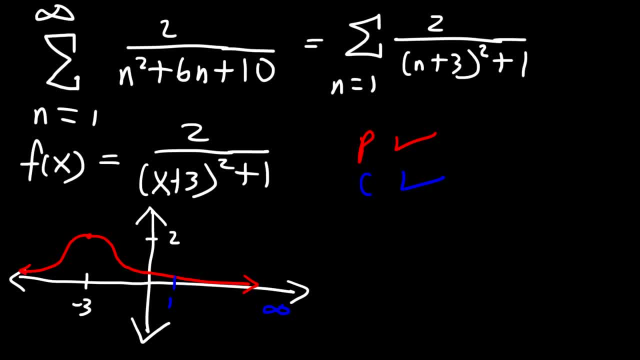 you could see that it's a decreasing function. it's positive, it's above the x-axis and it's continuous everywhere, from 1 to infinity. So we can use the integral test for that function. Now let's find the integral from 1 to infinity. 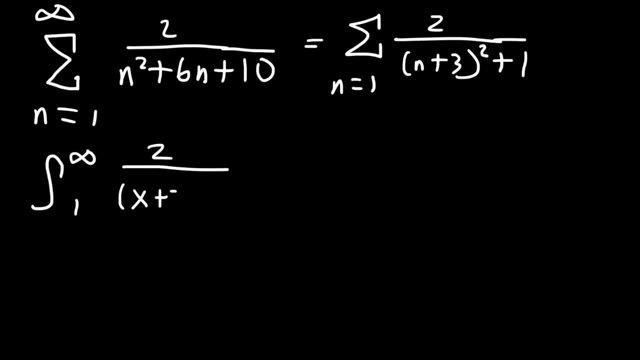 of the corresponding function, 2 over x plus 3, squared plus 1.. So for this problem we need to use trig substitution And if you see an integral with this generic formula or generic expression, this is equal to arctangent of x. 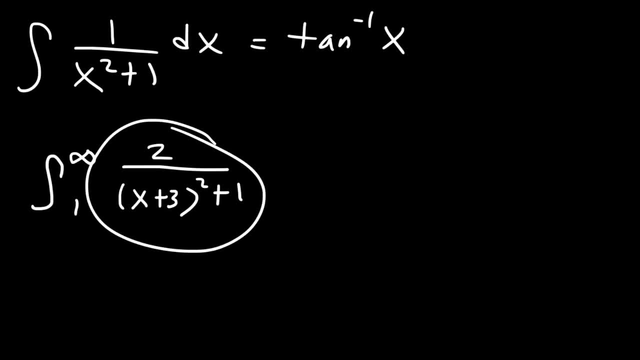 So this is going to be equal to something related to arctangent. So what we're going to do is replace x plus 3 with tangent theta. Now, if we differentiate both sides, we're going to get: dx is equal to the derivative of tangent, which is: 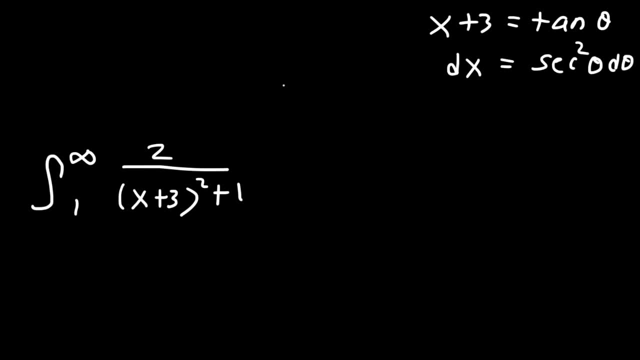 secant squared theta times t theta. So let's replace x plus 3 with tangent. So this is going to be tangent squared. And let's replace dx with secant squared theta. d theta 1 plus tan squared is equal to secant squared. 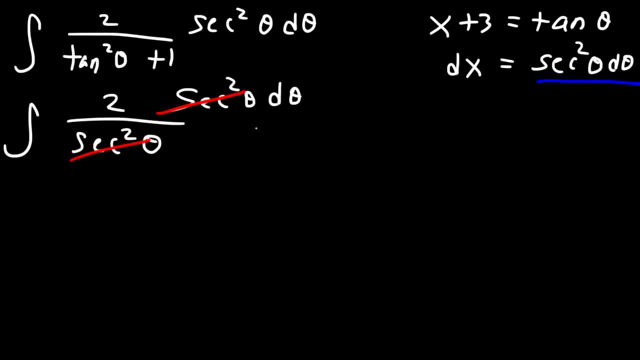 So now we can cancel these two expressions, And so this is going to give us the integral of 2d theta, which is 2 theta. Now, if x plus 3 is equal to tan theta, theta is arctan of x plus 3.. 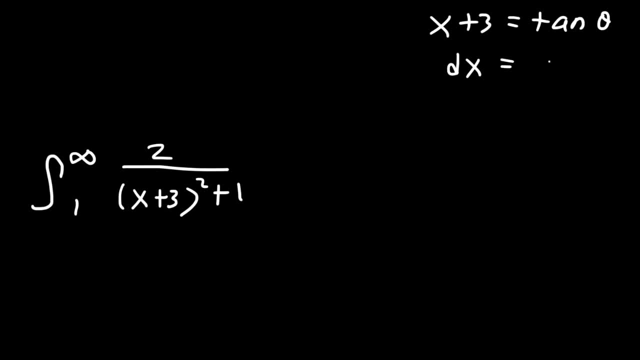 Now if we differentiate both sides, we're going to get: dx is equal to the derivative of tangent, which is secant squared theta times t, theta. So let's replace x with tangent theta, So this is going to be tangent squared. And let's replace dx with secant squared theta, d theta. 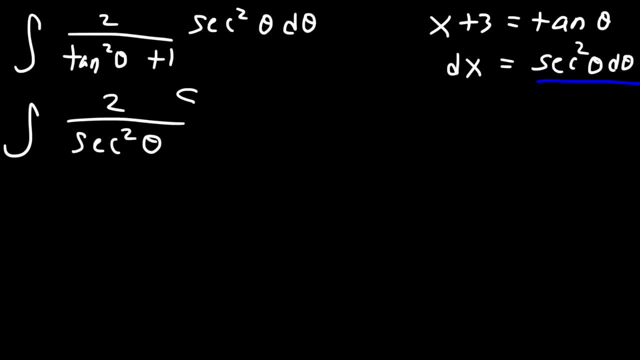 One plus tan squared is equal to secant squared, So now we can cancel these two expressions, And so this is going to give us, This is going to give us the integral of 2 d theta, which is 2 theta. Now, if x plus 3 is equal to tan theta, theta is arctan of x plus 3.. 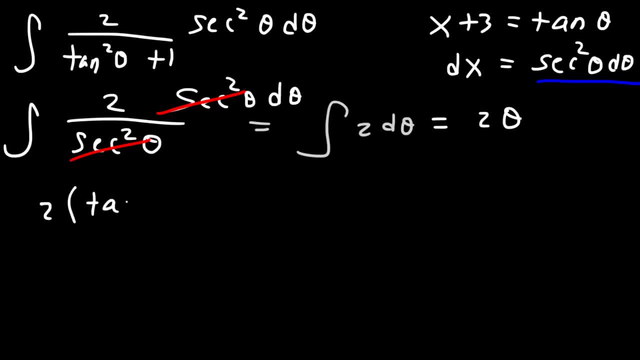 So we're going to have 2 times arctangent x plus 3.. Therefore, the integral from 1 to infinity of 2 divided by x plus 3 squared is going to be x squared. So we're going to do this. 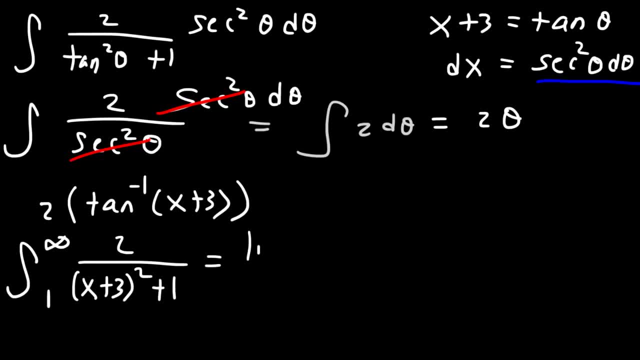 B squared plus 1, that's going to be equal to the limit as B approaches infinity for the integral 1 to B of the same expression. Let's not forget DX. So this is going to equal the limit as B approaches infinity, and then we're going to have 2 times. 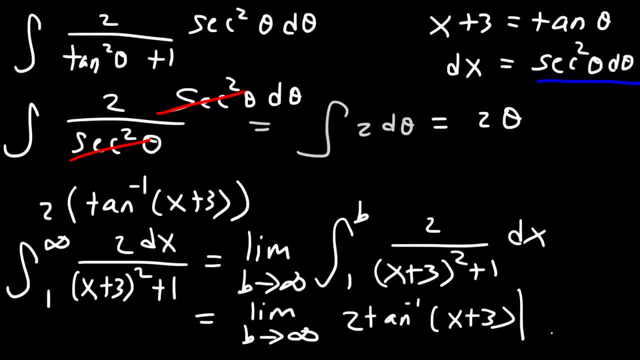 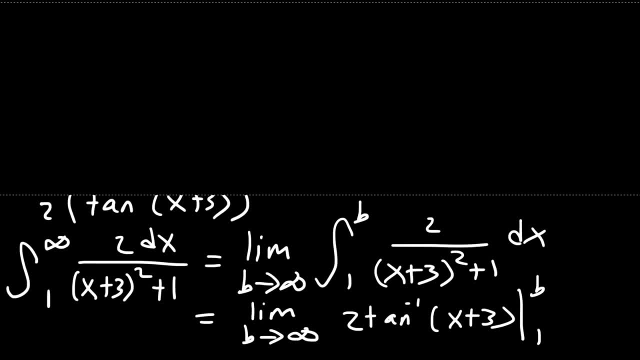 arc tangent, X plus 3, from 1 to B, And so that's going to be the limit as B approaches infinity, and then it's going to be 2 arc tangent, B plus 3, and then minus 2 arc tangent, and then it's going to be 1 plus 3, which is 4.. 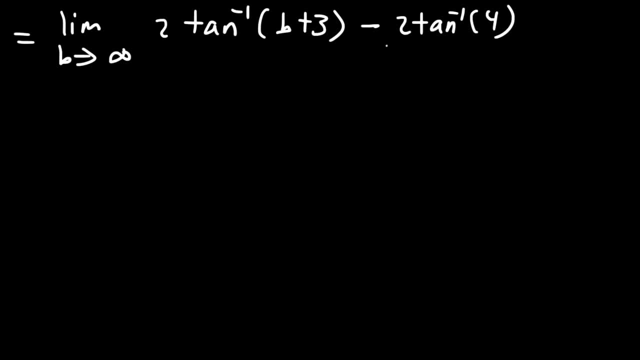 So infinity plus 3, that's going to be infinity. So what is arc tangent of infinity? If you draw a graph of arc tangent, it has two vertical asymptotes- not vertical asymptotes, but horizontal asymptotes- One at pi over 2 and the other at negative pi over 2.. 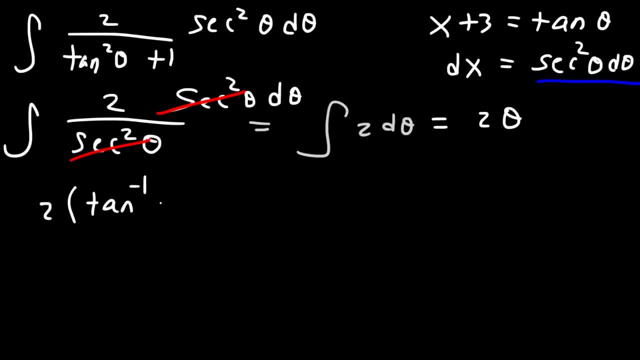 So we're going to have 2 times arctangent x plus 3.. Therefore, the integral from 1 to infinity of 2, divided by x plus 3, squared plus 1, that's going to be equal to the limit as b approaches infinity. 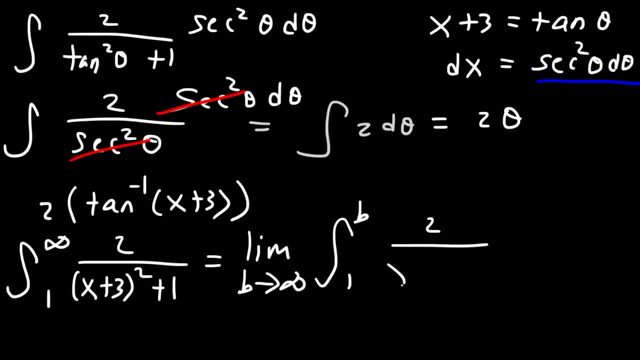 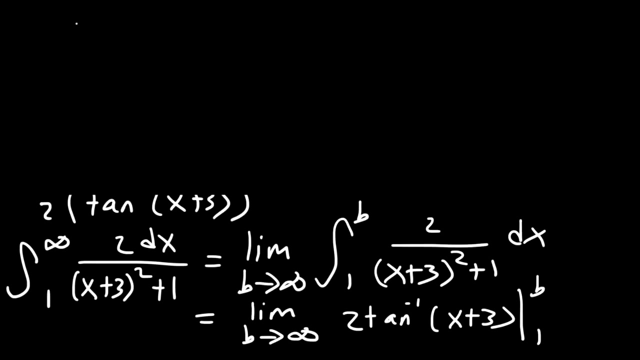 for the integral 1 to b of the same expression, And let's not forget dx. So this is going to equal the limit as b approaches infinity, And then we're going to have 2 times arctangent x plus 3 from 1 to b. 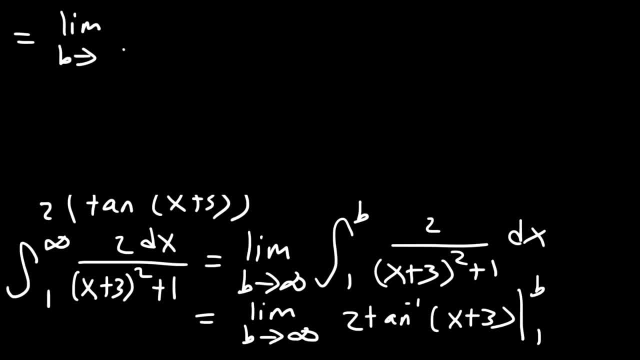 And so that's going to be the limit as b approaches infinity, And then it's going to be 2 arctangent, b plus 3, and then minus 2 arctangent, And then it's going to be 1 plus 3, which is 4.. 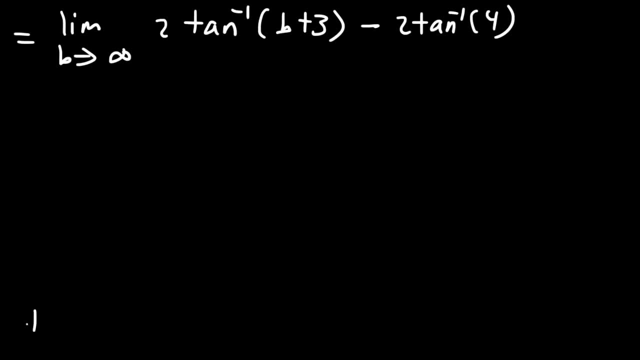 So infinity plus 3, that's going to be infinity. So what is arctangent of infinity? If you draw a graph of arctangent, it has two vertical asymptotes- Not vertical asymptotes, but horizontal asymptotes- One at pi over 2 and the other at negative pi over 2.. 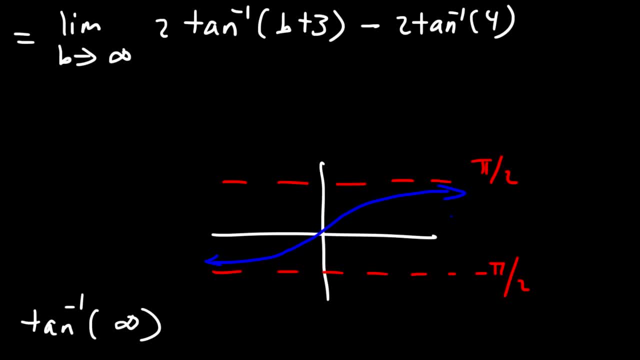 And the graph looks something like this: So as x approaches positive infinity on the right, the y value will approach pi over 2.. So arctangent of infinity is pi over 2.. Now, if you put your calculator in radian mode, 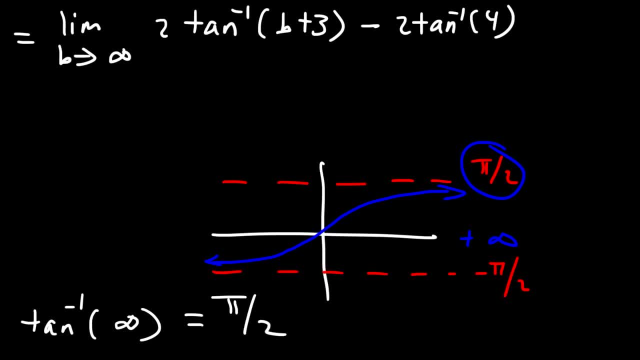 and if you type in arctangent of 1000, it will give you 1.5.. 7,, which is approximately pi over 2.. Or if you put it in degree mode and type in arctangent of 1000,. 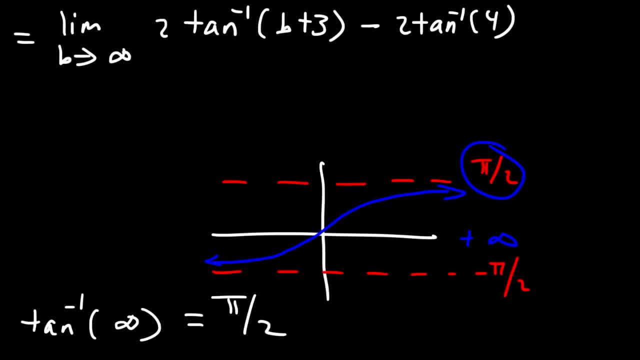 it will give you 89.9, which is close to 90 degrees, which is about pi over 2.. So this part, as b goes to infinity, that's going to converge to pi over 2.. So this expression pi over 2 minus. 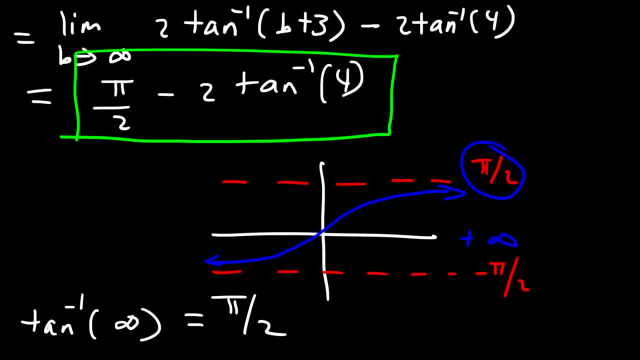 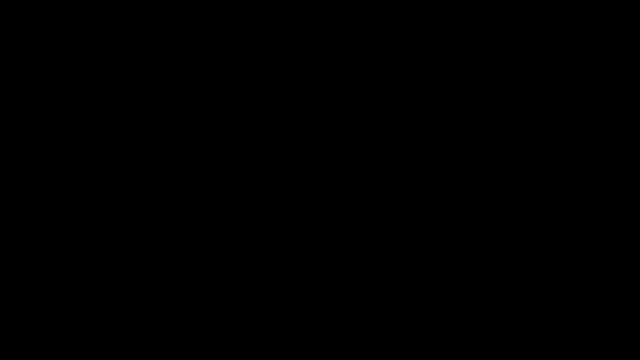 2 arctangent of 4,. it has a finite value, which means that the integral converges, And so if the integral is convergent, then the series will also converge, And that's the final answer, Thank you, Thank you. Thank you. 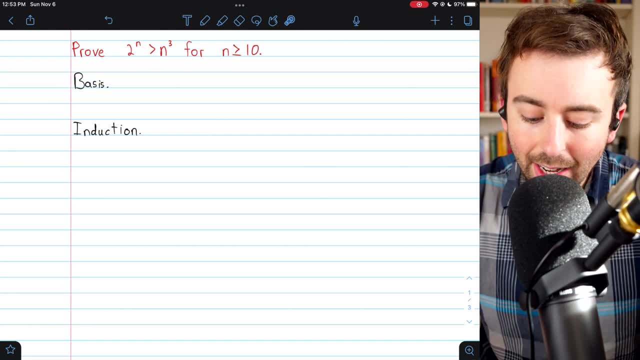 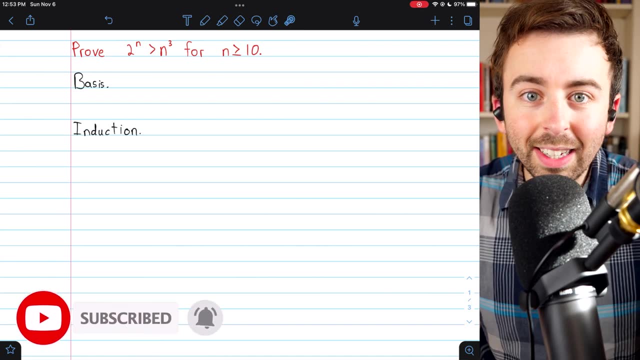 We're going to prove that 2 to the n is greater than n cubed for all n greater than or equal to 10.. Since this is a statement about all positive integers, you might think to try a proof by induction, and that's exactly what we'll do here. There are a few steps to this induction proof. 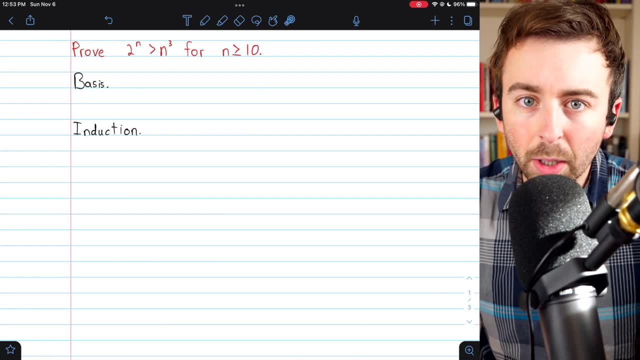 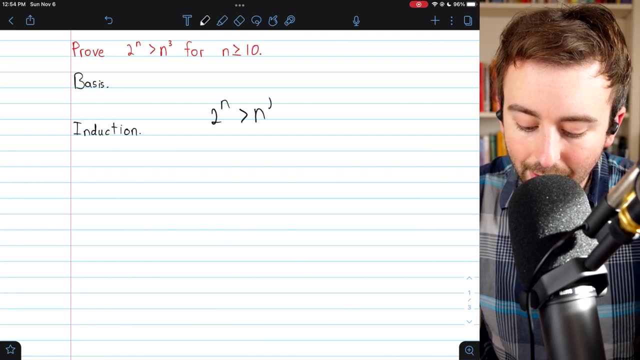 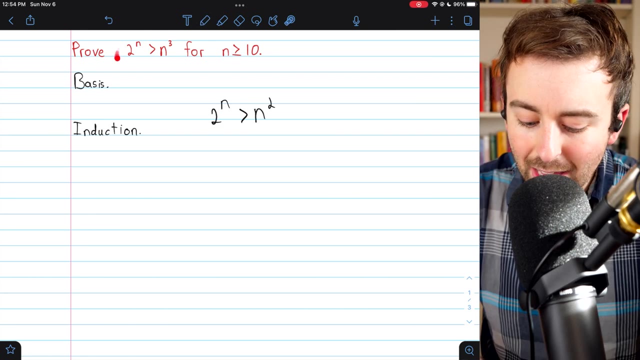 but it is fairly straightforward. It's really similar to another result. we proved previously that 2 to the power of n is greater than n squared. I'll leave a link in the description to my lesson proving this result. If you check that out, you should try this one yourself. 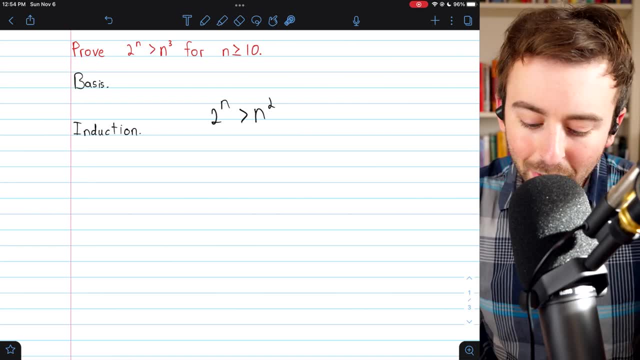 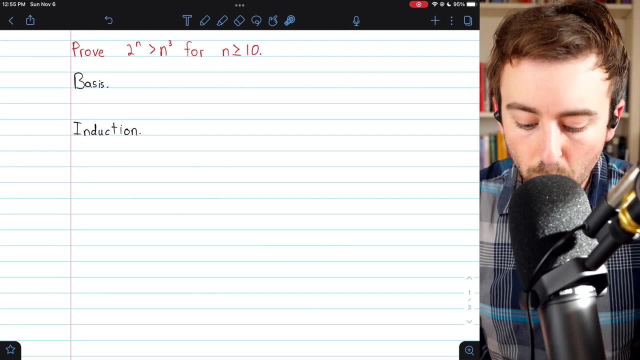 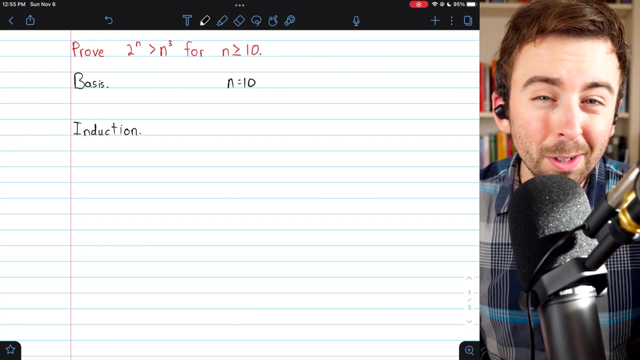 because, like I said, the strategies are really similar With. that said, let's get into this proof. We begin with our basis step, showing that our statement is true for the first number of interest. In this case, the first number of interest is: n equals 10.. For numbers, 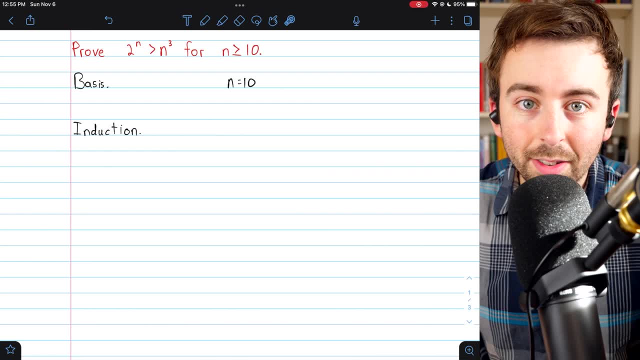 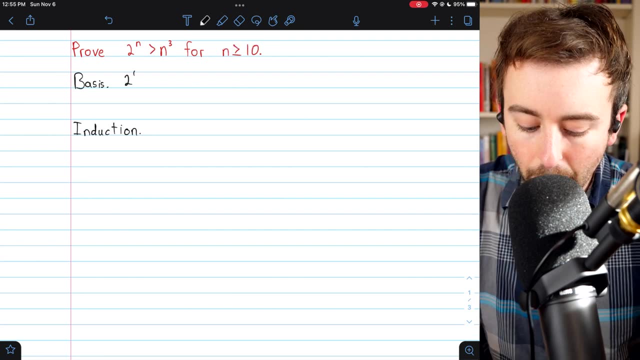 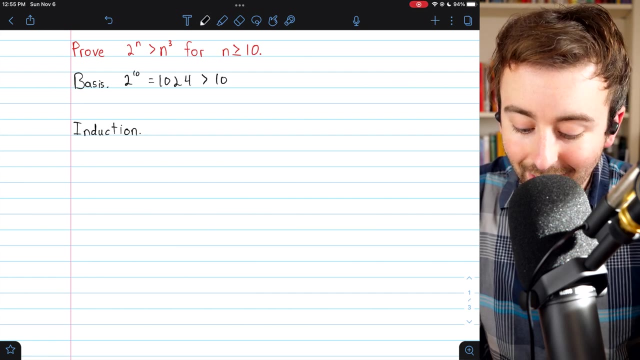 before 10,. this result is mostly false. So we've got to wait until n equals 10 for it to hold. So we'll say: let's look at 2 to the power of 10.. This is equal to 1024,, which is greater than. 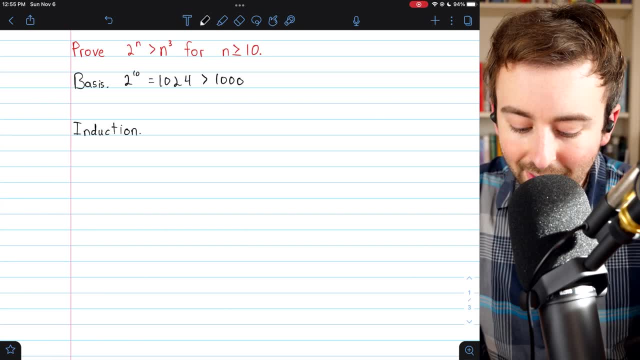 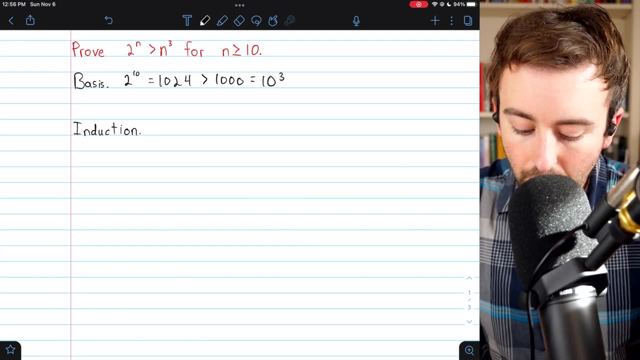 1,000, certainly. And what's important about 1,000 is that 1,000 is n cubed when n equals 10.. So this is equal to 10 cubed. So we see that 2 to the 10.